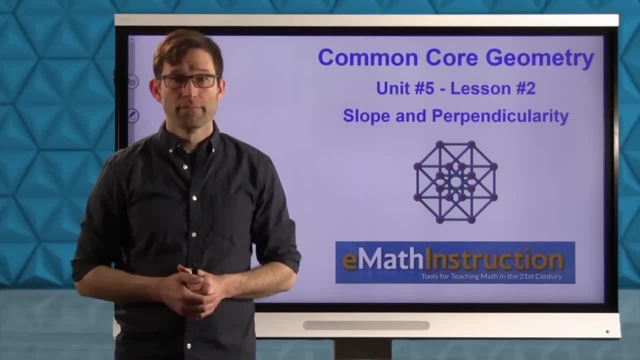 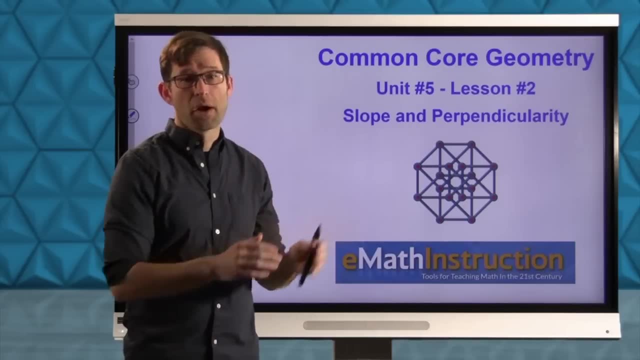 same slope, and if they have the same slope they'll be parallel. Alright, Yeah well, whatever. So it's an equivalence thing. Equal slopes means parallel. basically, Today we're going to look at the relationship that occurs between the slopes of lines that. 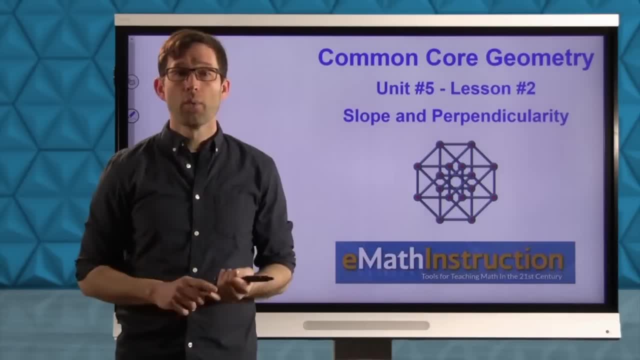 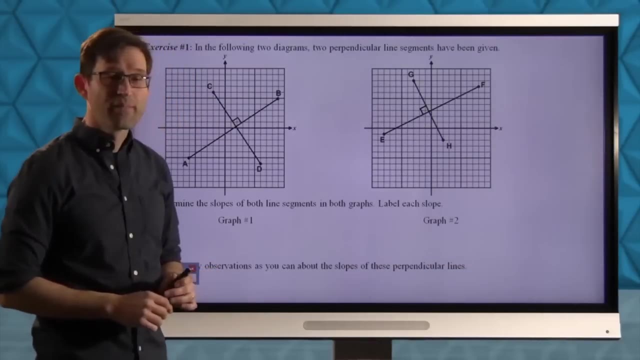 form 90 degree angles with one another, And of course, those are critical when you look at right triangles, rectangles, squares and a variety of other geometric figures. So let's jump right into it and let's see if we can discover that relationship. Alright, now in. 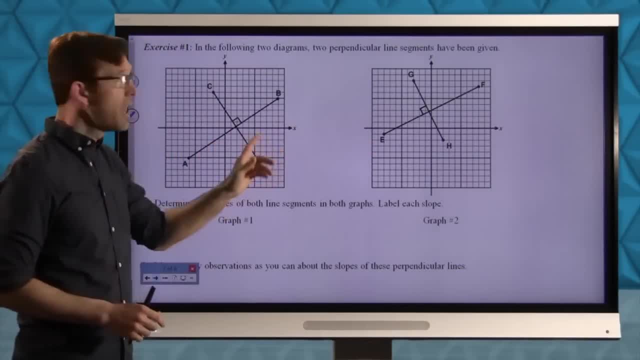 exercise 1. what we've got is: we've got two graphs, okay, And in both situations I've drawn line segments that are perpendicular to one another. Now, in exercise 1, we've got two graphs, okay, And in both situations I've drawn line segments that are perpendicular. 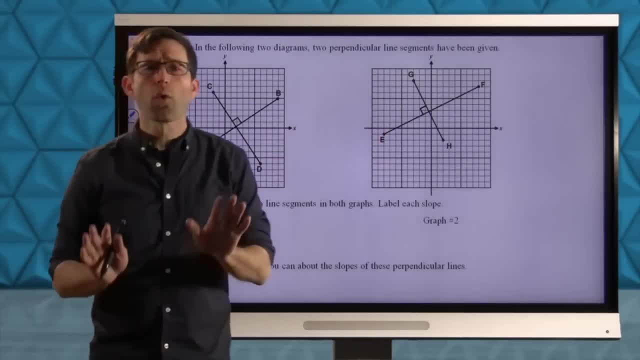 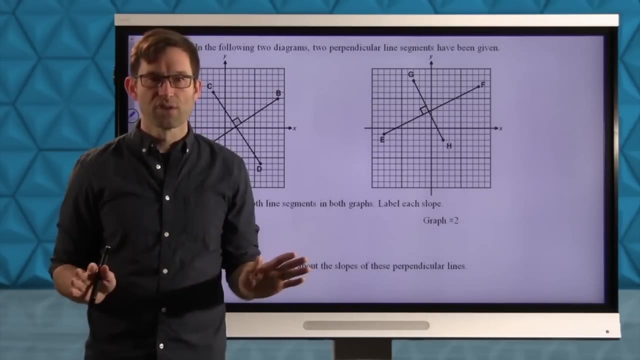 to each other. And what I'd like to do is I'd like to just graphically, graphically, determine the slopes of all the line segments involved. Okay, So what I say we do is we do the first slope of letter A together and then have you do all the rest of the slopes. 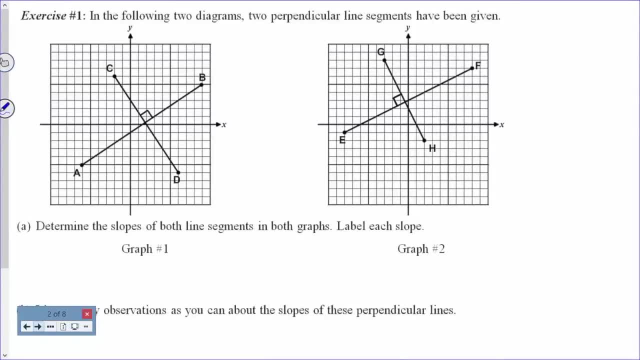 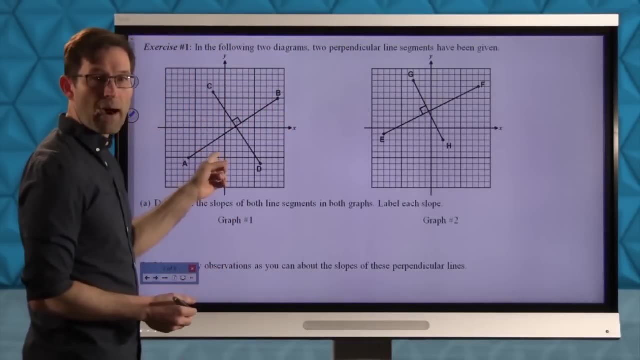 on your own. So let's jump into it. Exercise number one: In the following two diagrams, two perpendicular line segments have been given Letter A. determine the slopes of both lines In both graphs. label each slope. Alright. so together let's talk about line. 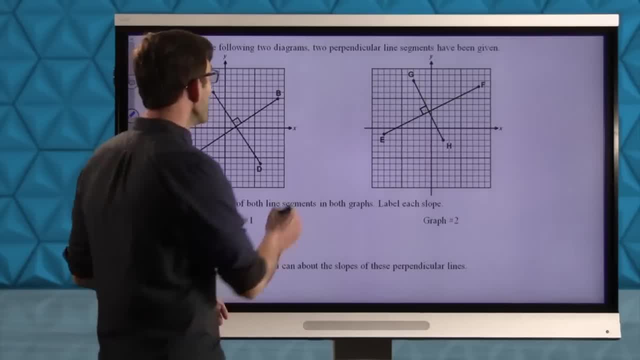 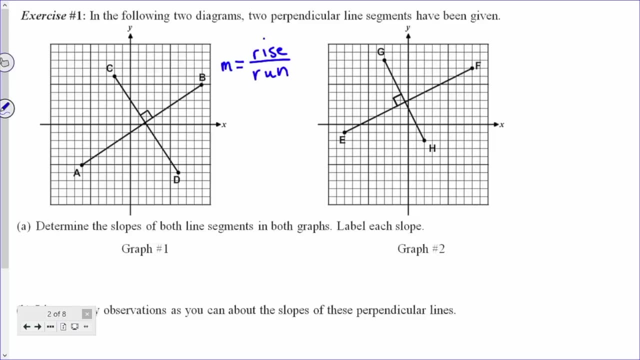 segment AB and find its slope graphically. Remember slope right will be rise divided by run, the ratio of rise to run. So if we look at line segment AB and we pull off that point and then we look for another one, that's nice, and maybe another one that's nice, etc. 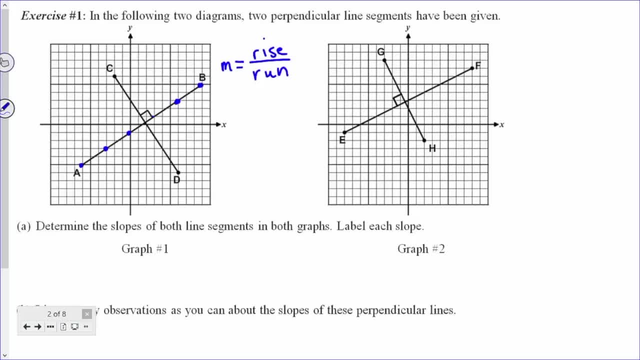 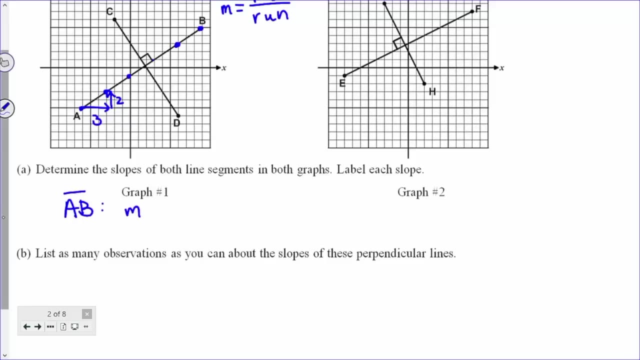 right, It doesn't have to be nice points, but nice points are nice, if you know what I mean. right, What we see is that we run three units for a rise of two units every time. So for AB I would say that the slope is two-thirds, And actually let's do CD together as well. 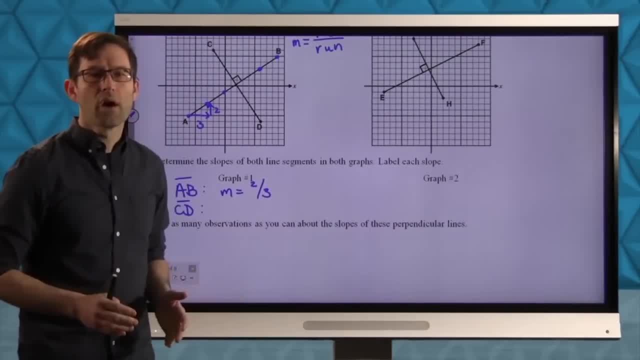 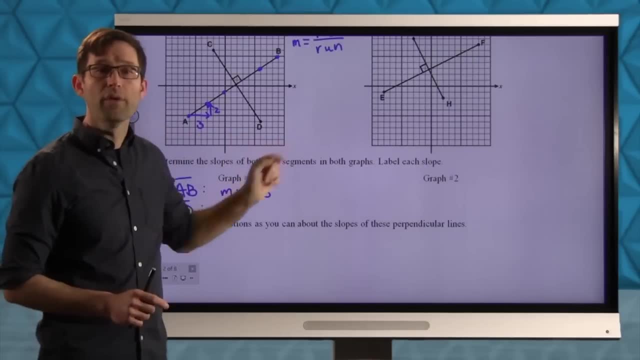 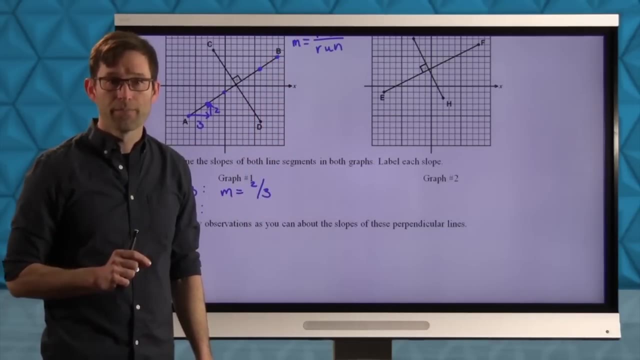 Alright, And the reason that I want to talk about CD right is that CD is the slope of the line segment CD. you should immediately look at and say, as we read this graph moving left to right, CD is going down And therefore it has to have a negative slope to it. A negative slope. 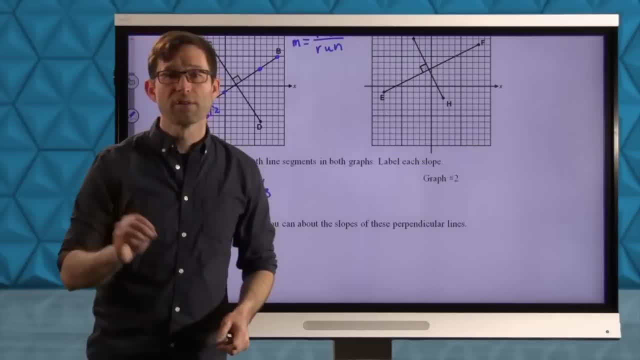 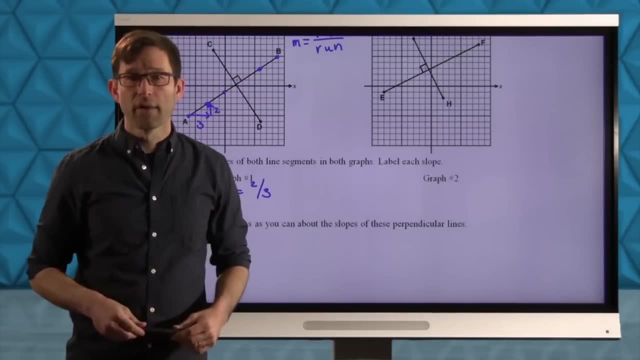 Now with the slope formula you don't have to worry about that. that whole y2 minus y1 divided by x2 minus x1.. Plenty of practice with that. today You don't have to worry about positive, negative. it'll come out in the calculation When you're doing it graphically, you literally. 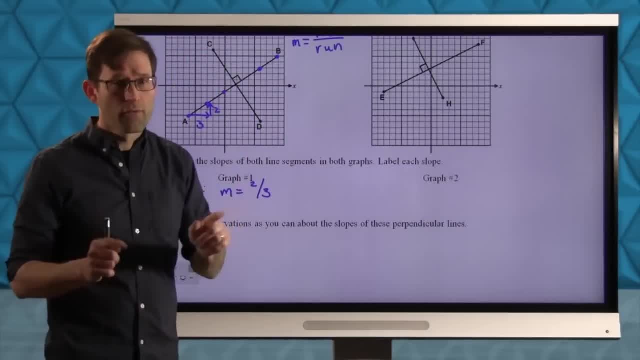 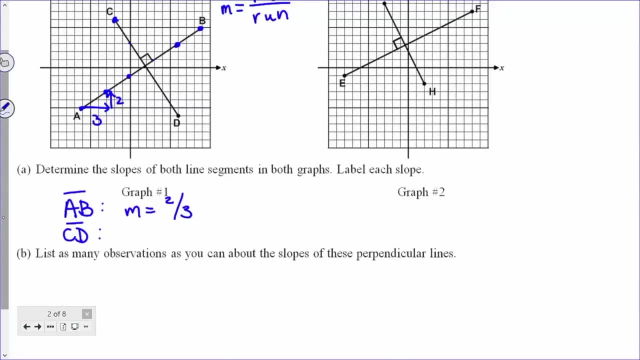 have to look at CD and go: well, that thing is going down. therefore it has a negative slope. Let's take a look at CD. Same kind of idea. Try to find some nice points. There's a nice one, a nice one, a nice one, etc. Alright, And what I see is that for every two units, 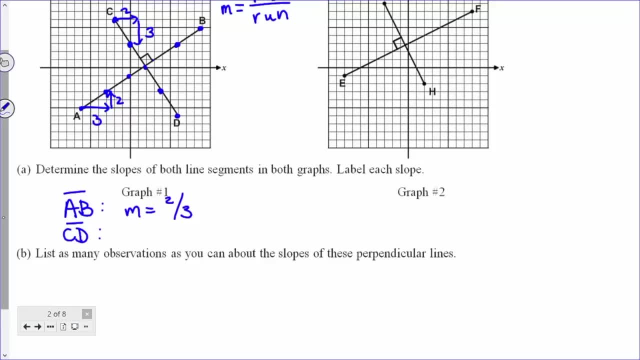 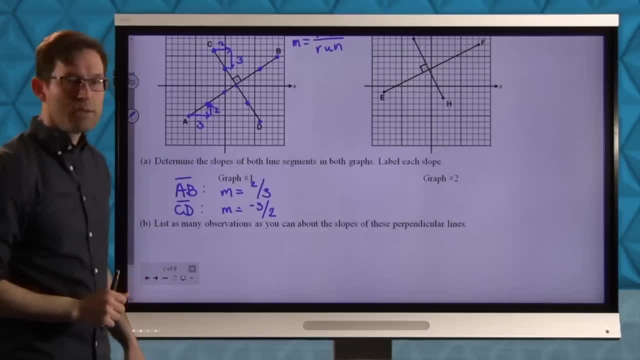 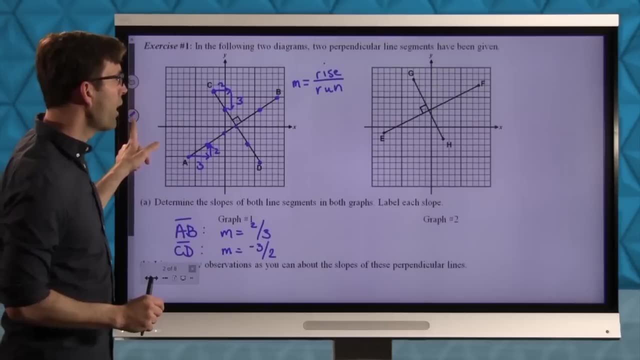 that it runs. it actually falls three units. So the slope of CD will be negative three-halves. So the slope of AB is positive 2 thirds and the slope of CD is negative 3 halves. Alright, why don't you go ahead? 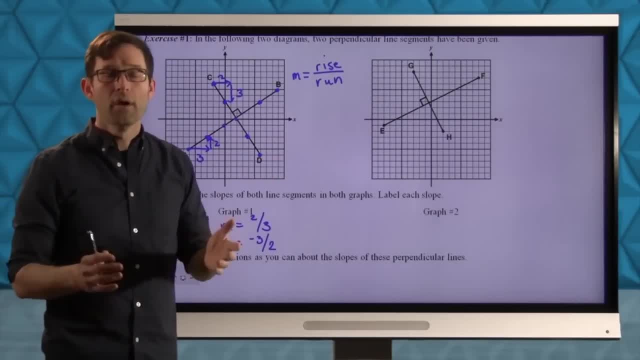 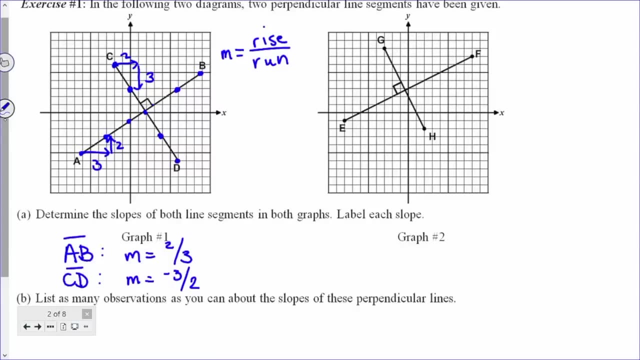 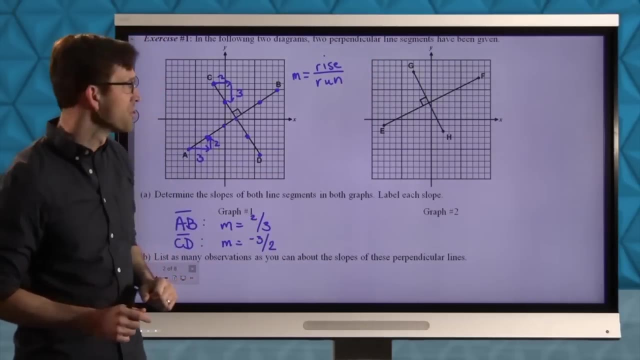 and do the two slopes from this particular graph. Pause the video and take as much time as you need. Alright, let's go through, and maybe what I'll do is I'll work them out kind of up top here and then we'll put them down in the results down here. Let's take a look. 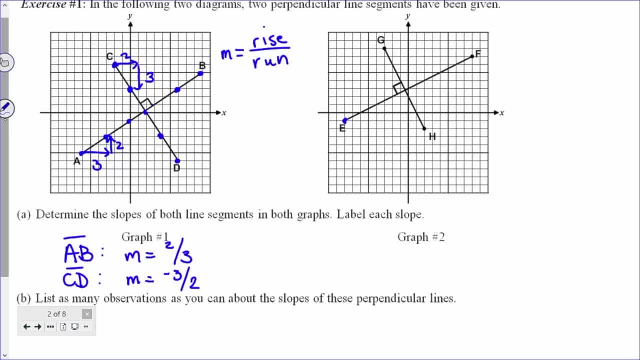 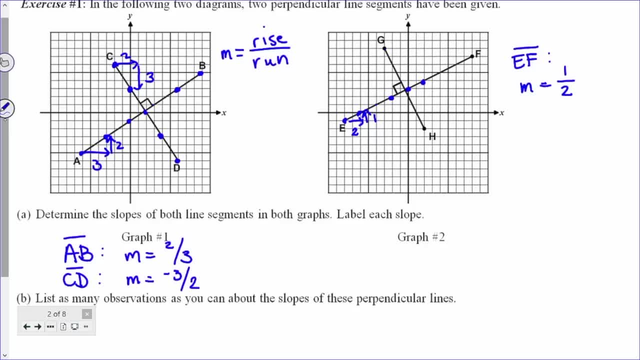 two Now, just like before. GH certainly looks like it's got a negative slope. Doesn't just look like it, it does A little bit trickier. for every run of one it's dropping two. So for GH, right, its slope will be negative. 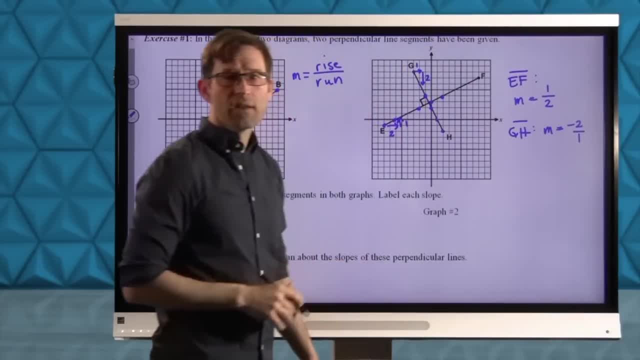 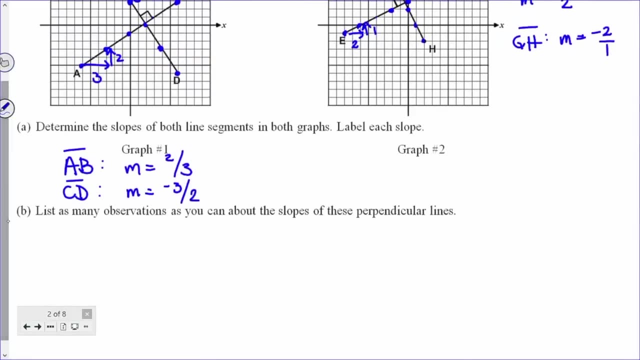 2 over 1 or just negative 2, but I like to keep it as negative 2 over 1 for right now to see this relationship. So let me, let me bring these up and write them right down here so that we can compare contrast etc. For EF, we see a slope of positive one-half and for GH, 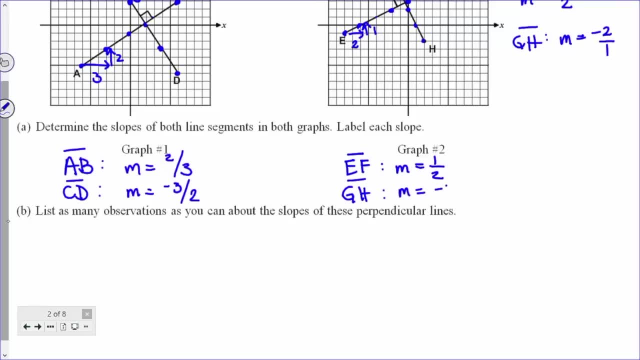 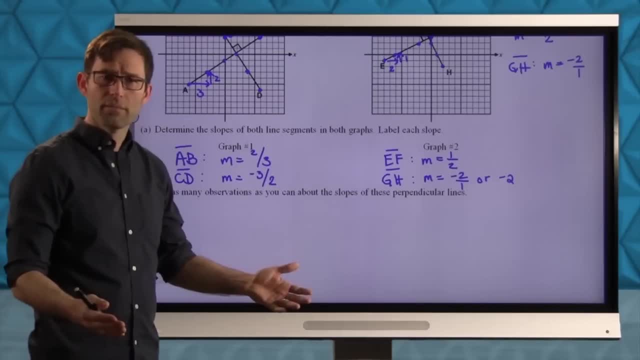 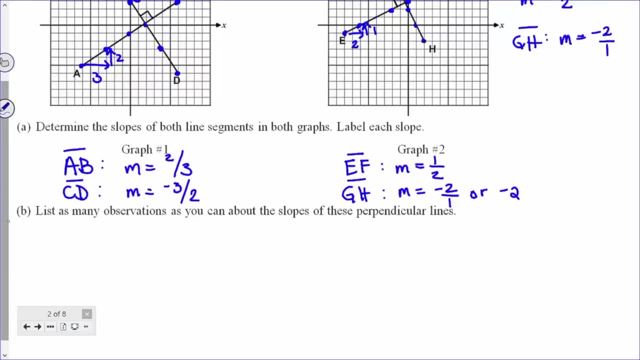 we have a slope of negative 2 over 1, or just negative 2.. Alright, now what we'd like to do is see if we can kind of deduce a pattern here. alright, Letter B says: list as many observations as you. 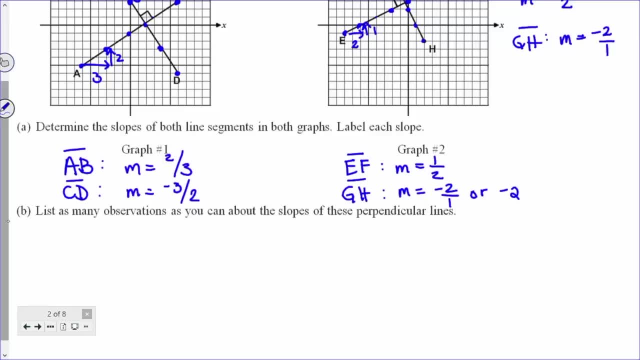 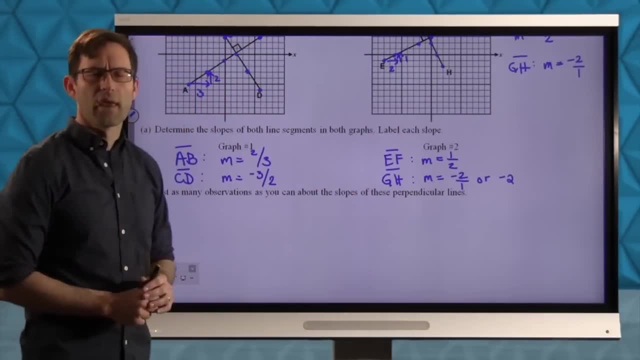 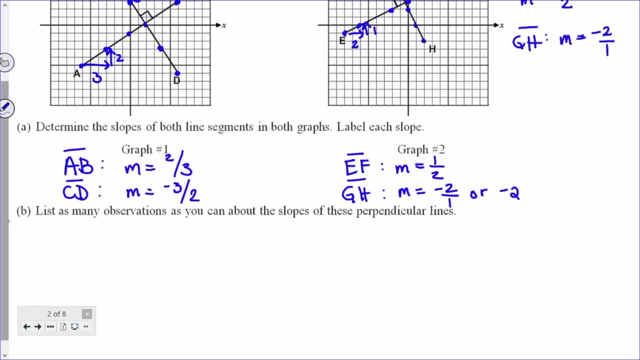 can about the slopes of these perpendicular lines. Alright, now again, what I want you to do is kind of compare these, think about them, compare these, think about them and write down anything. you can Take a few moments, Alright. well, hopefully one thing is pretty. 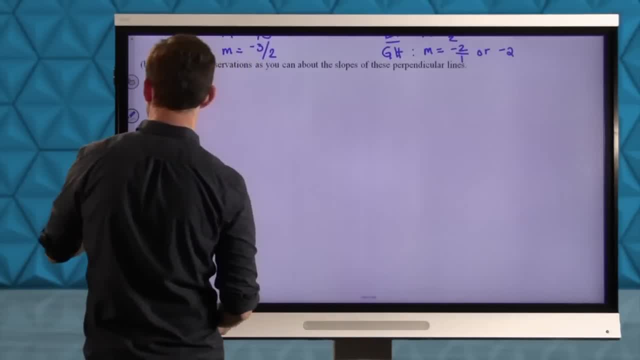 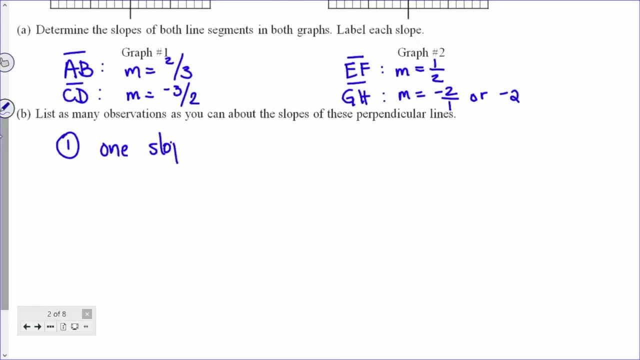 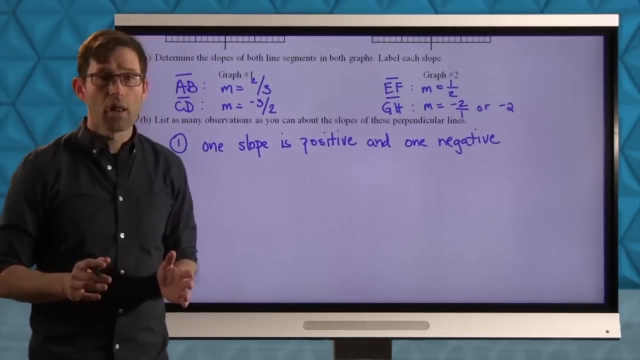 obvious. Extend the page a bit, bring it back down. So observation one that I would make is: one slope is positive and one negative, Or you could say they have opposite signs right Now. it will always be true as long as you don't have vertical or horizontal lines. 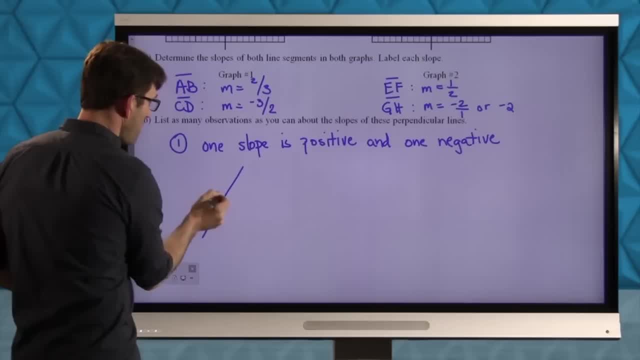 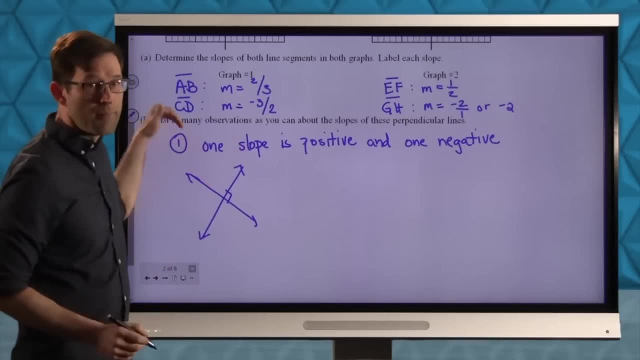 two lines will be perpendicular. Well, one of them, if it's got a positive slope, the other one's got to have a negative slope. There's just no getting around that, right, If one of them's going up, the other one has to go down. The other observation is a little. 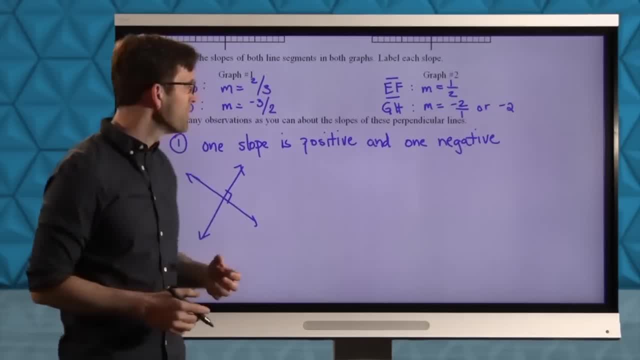 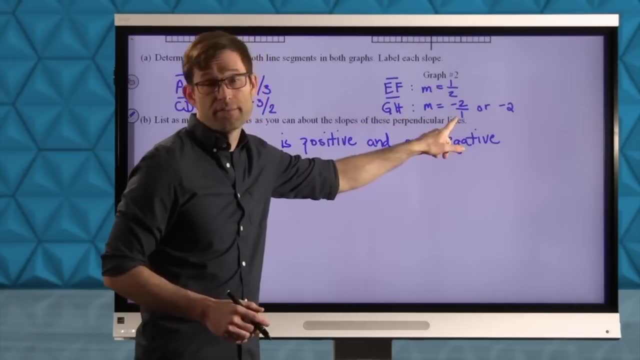 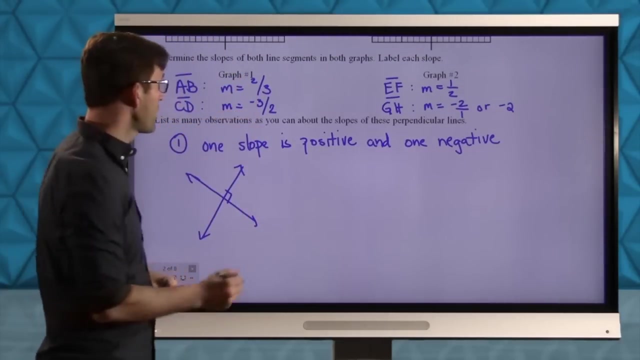 bit trickier, especially like trickier, to kind of verbalize. But notice, forgetting about the negative. for a second, Two-thirds and three-halves, One-half and two-firsts, or one over two, two over one, two over three, three over two, Okay, 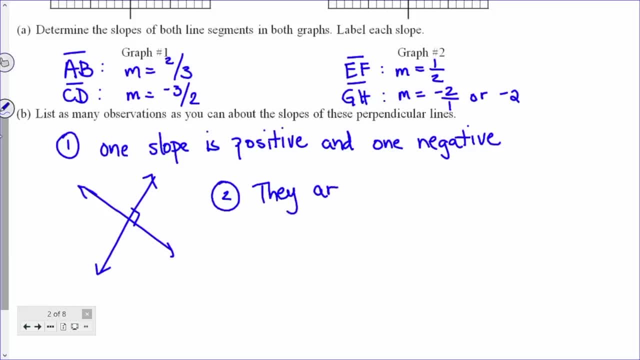 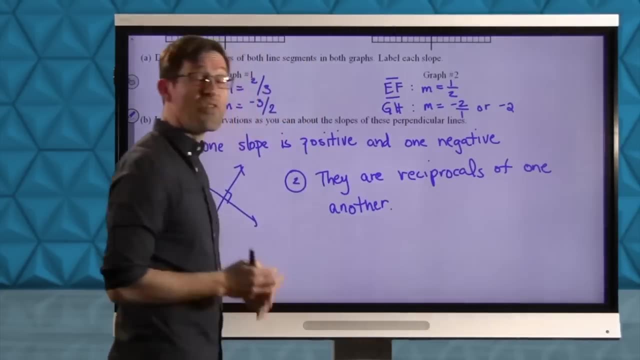 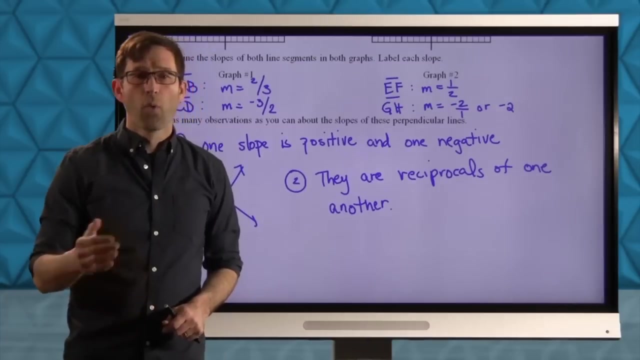 They are. the fancy term is reciprocals. Actually they aren't reciprocals of one another, but their absolute values are Alright. Reciprocals are numbers like, let's say, four-thirds and three-fourths, Seven-halves and two-sevenths. right, It's when you take a fraction and you 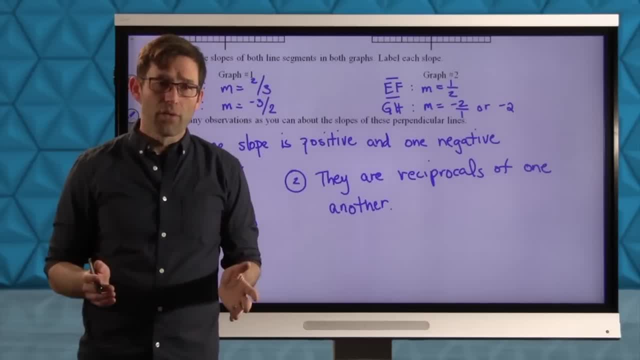 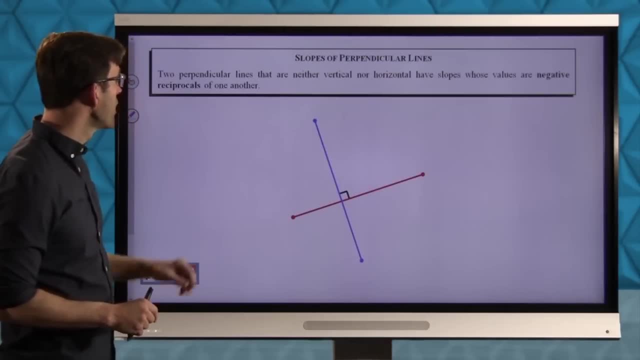 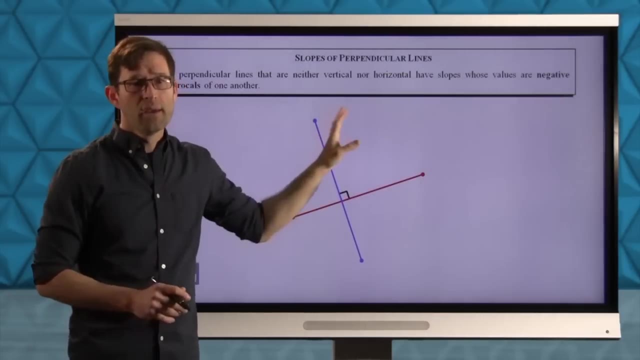 flip it, so to speak. So altogether, though right altogether, we can summarize this in the following slide: Okay, Two perpendicular lines that are neither vertical nor horizontal, and when we have our lesson on vertical and horizontal lines, it'll make a lot more sense. 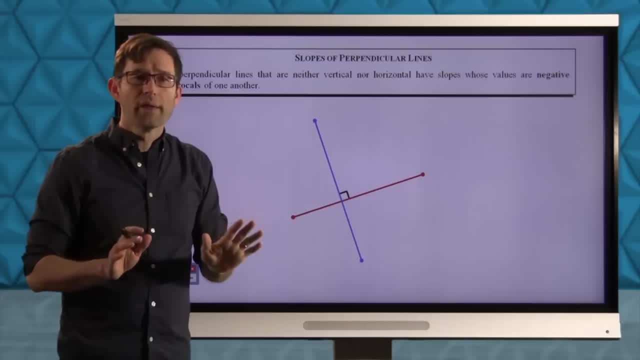 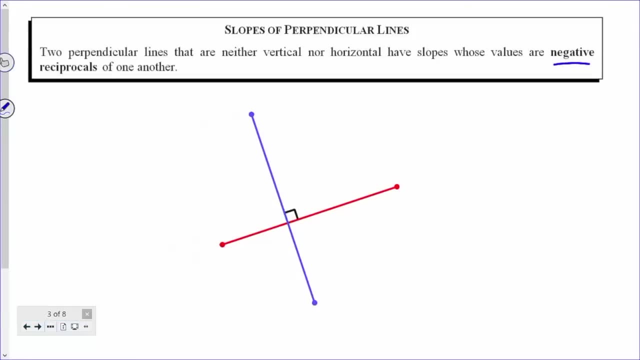 why I've got to keep putting this in. But for right now, two lines that are neither horizontal nor vertical, that are perpendicular, will have slopes that are negative reciprocals Of one another, Negative reciprocals of one another. So, for instance, if I've got this: 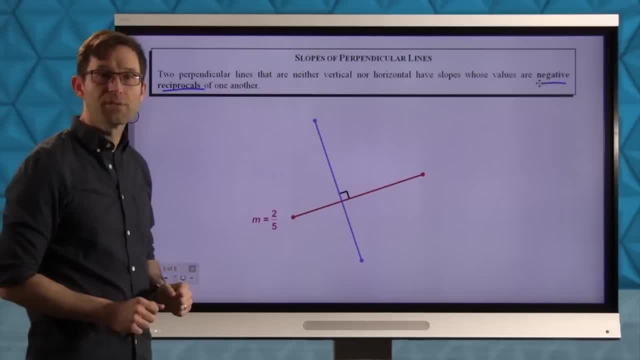 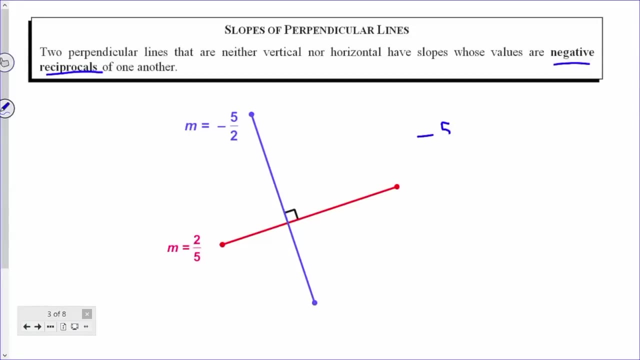 red line segment. let's say its slope was two-fifths. Then this blue line segment that's perpendicular to it, would have a slope of negative five-halves. Okay, Some math teachers will give you another test. They'll say that two lines are perpendicular if the product 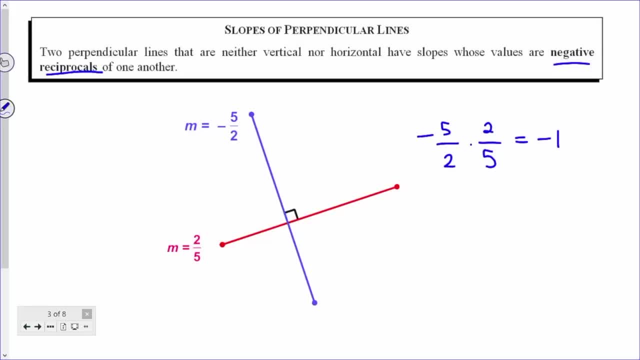 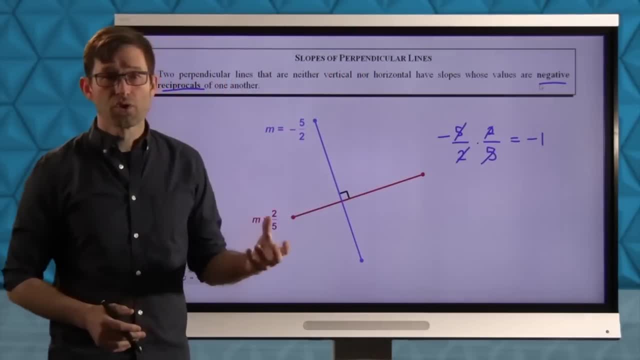 of their slopes is equal to negative one. Right, Notice all of those kind of cancel out, And that's absolutely true. It was true in the first case where we had a, I think, a slope of two-thirds times a slope of negative. 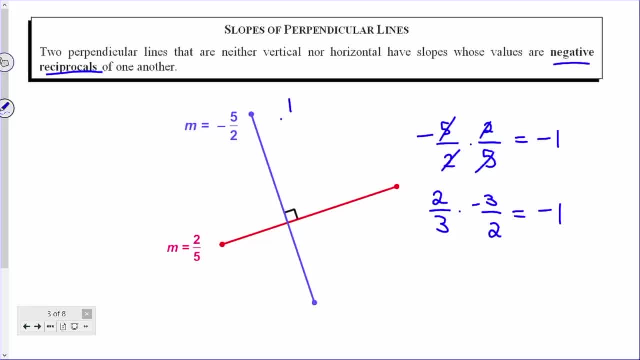 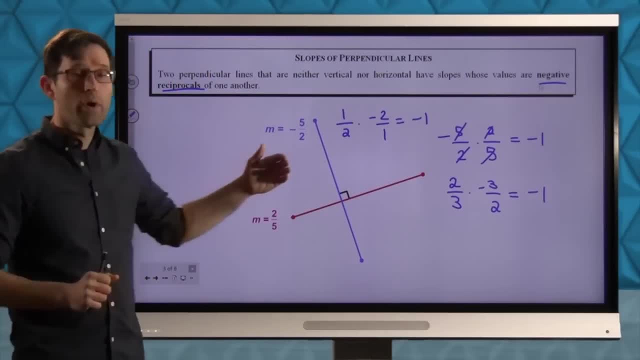 three-halves, That equals negative one. Even when we had a slope of one-half and a slope of negative two, that has a product of negative one. But the technical wording on it is that two lines will be perpendicular if their slopes are negative reciprocals of one another. Alright, 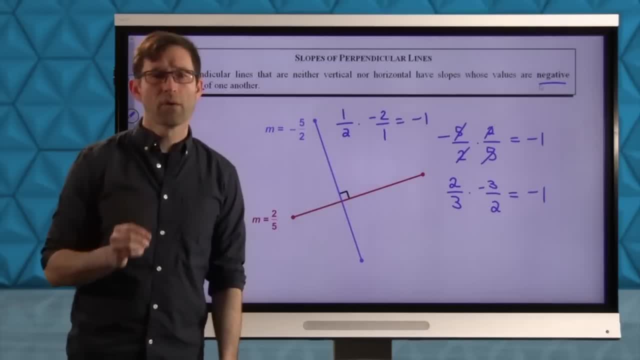 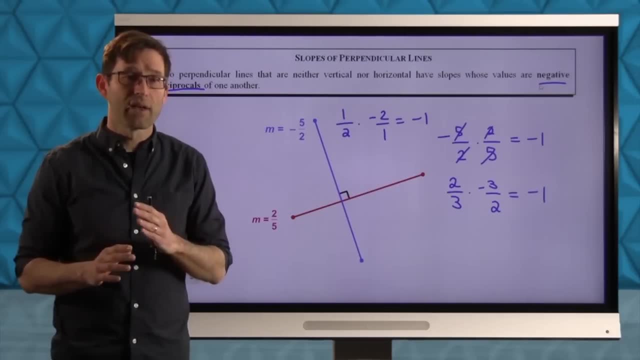 Now that's a much, much more difficult relationship than what we saw with parallel lines, which is, hey, if they're parallel, they have the same slope- Okay, But perpendicularity is about those lines having about as opposite slopes as they can be. if you think about 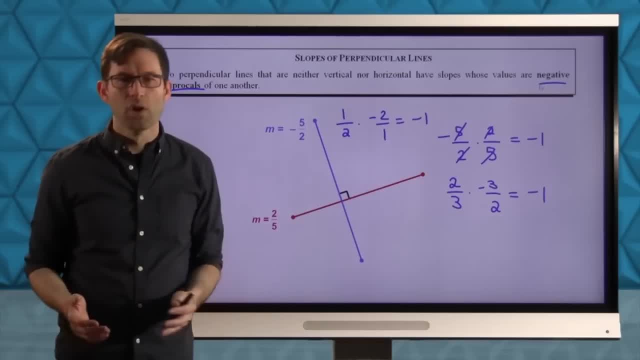 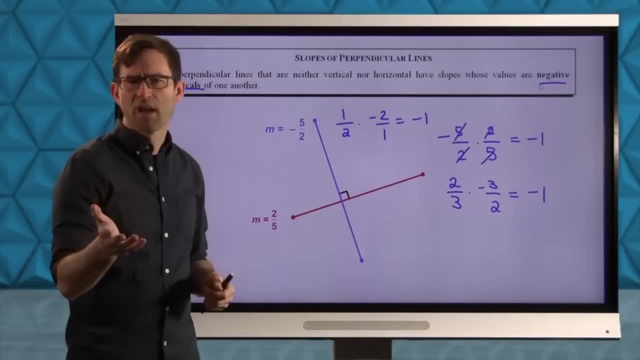 it Now, you don't want to say it that way, You don't want to say, oh, if they have opposite slopes, Because the word opposite in math is a very loaded term. You know, if I said, hey, what's the opposite of five? you might say negative five, Or you might say one-fifth. 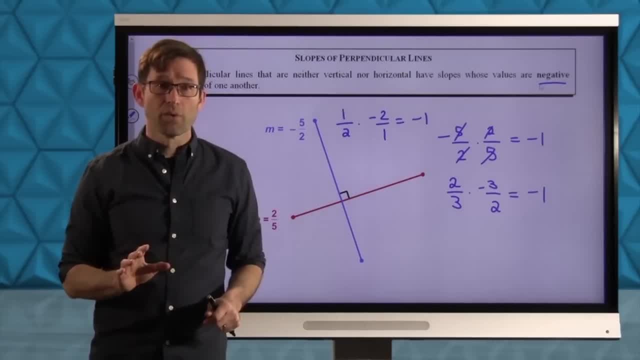 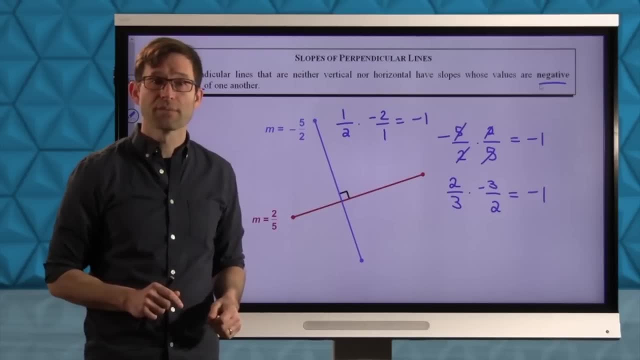 Right. So basically, negative reciprocals means that if one's negative, one's positive, And if one is two-thirds, the other one is negative three-halves. Alright, So now let's use this relationship for the rest of the lesson to both do some problem solving and a little. 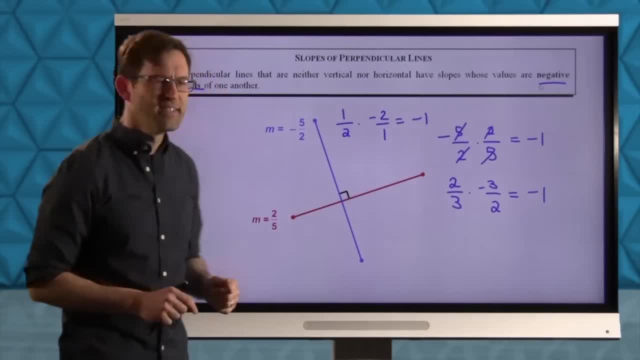 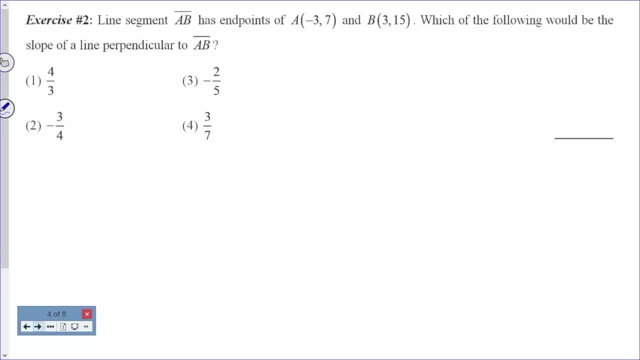 bit of what's called coordinate geometry proof. Alright, let's do it. Okay. Exercise number two: Line segment AB has endpoints of negative three-seven and three-fifth. Which of the following would be the slope of a line perpendicular to AB? Okay Now. 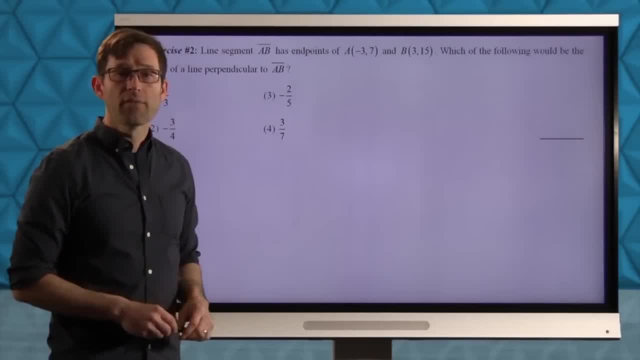 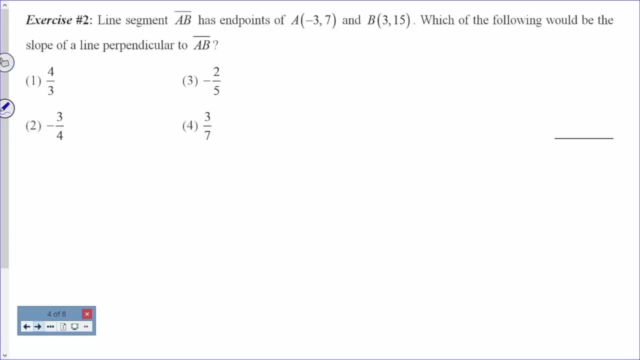 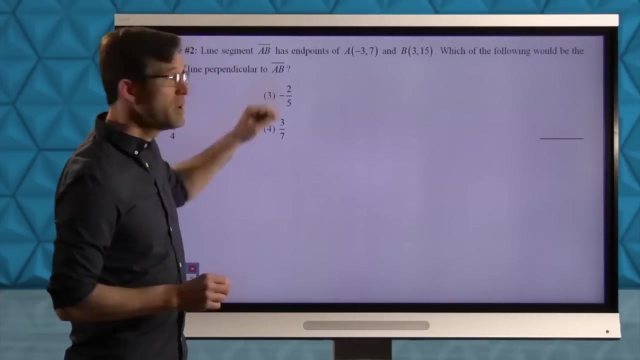 you know everything you need to know to solve this problem now, So I'd like you to take a few minutes and take a shot at it. Okay, Well, let's work on it. We know that any line that is perpendicular to AB will. 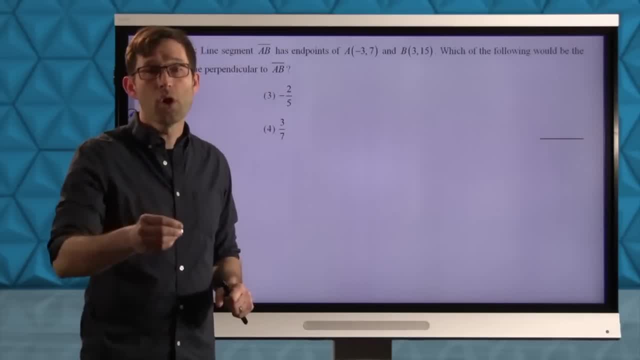 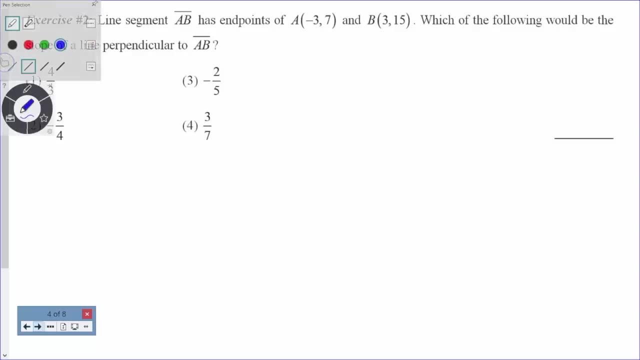 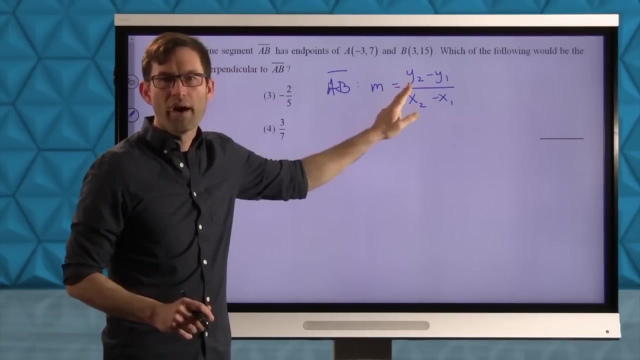 have a slope. that is the negative reciprocal of negative three-seventh. So now take a look at the answer page. So this is the beginning of class A. Okay, Alright, Then we have b. we're gonna take the change in y divided by the change in x. Remember as well, it doesn't matter which. 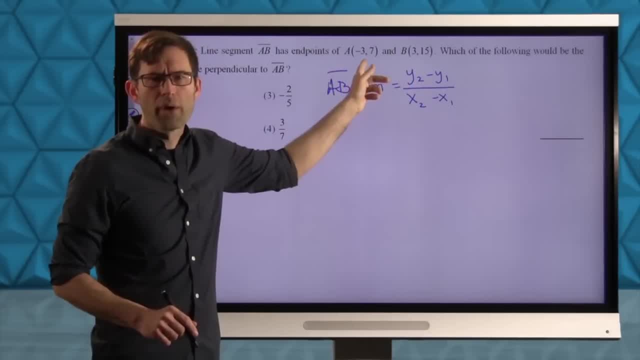 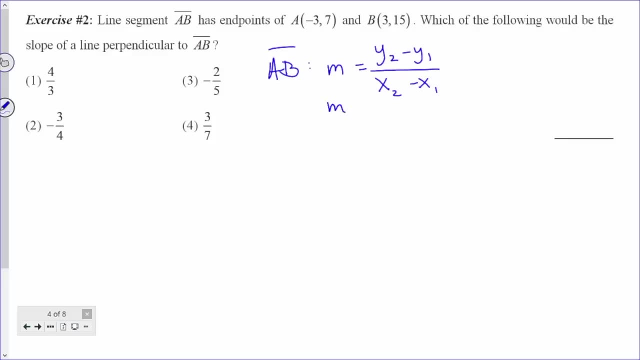 one you call x1, y1 and x2, y2, but I'll probably always stick with the first one being x1, y1 and the second one being x2, y2.. So for a, b whoops, let me move that. 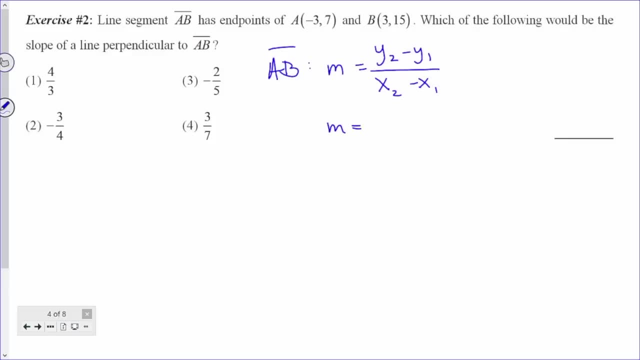 m a little bit farther down. For a, b, I can say that the slope is 15 minus 7 in the numerator. Watch out: in the denominator that's going to be 3 minus a negative 3.. So we'll have 8 sixths in the numerator, and it's always a good idea. 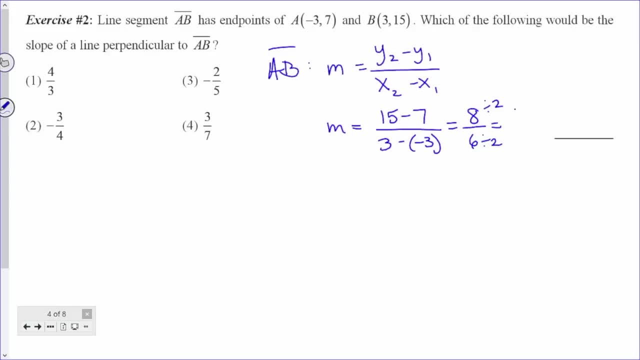 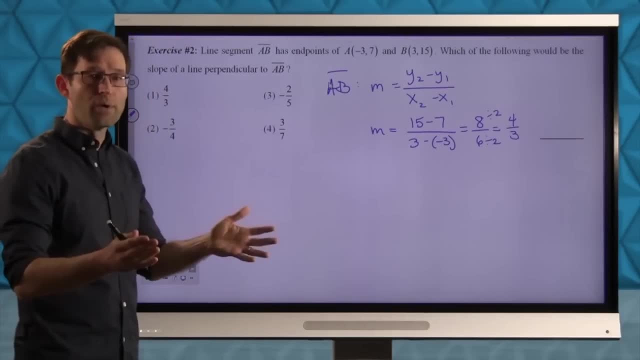 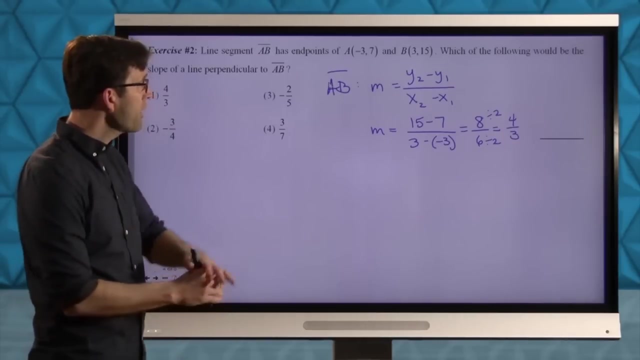 when you can reduce a slope to reduce a slope. So the slope of a- b is 4 thirds. Now, as always, as always, if you're doing a multiple choice question, be very, very careful about getting a result and thinking: I'm done Right, hey, I got 4. 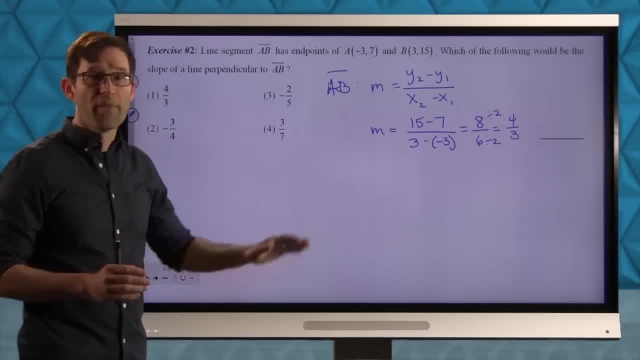 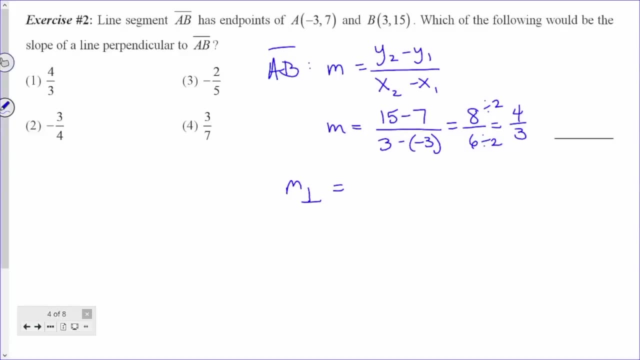 thirds. the answer is number 1.. But the answer is not number 1.. That's the slope of a- b, But the slope then that's going to be 4 thirds. So if you're doing a question that would be perpendicular to a- b, not the slope but the line segment. 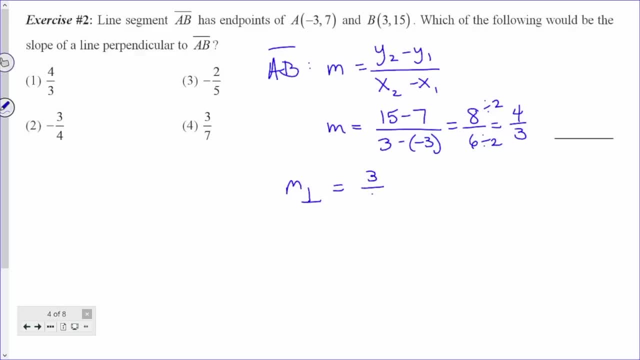 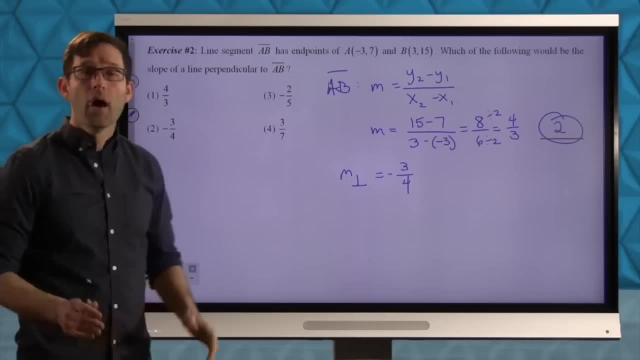 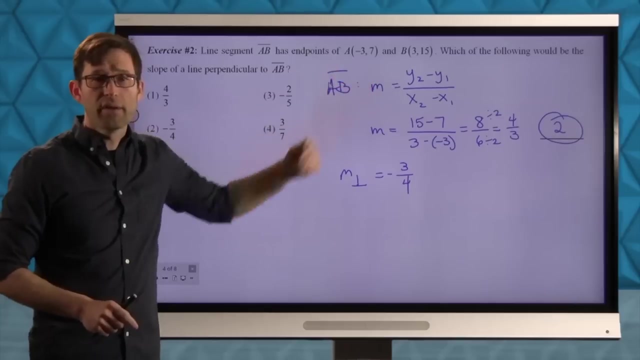 right would be the reciprocal of 4 thirds, which is 3 fourths, and the negative reciprocal, So that's choice 2.. All right, a very straightforward problem that requires two pieces of knowledge. Piece number 1, how do you calculate the? 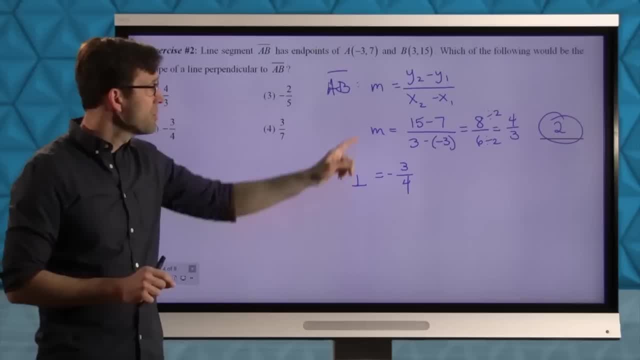 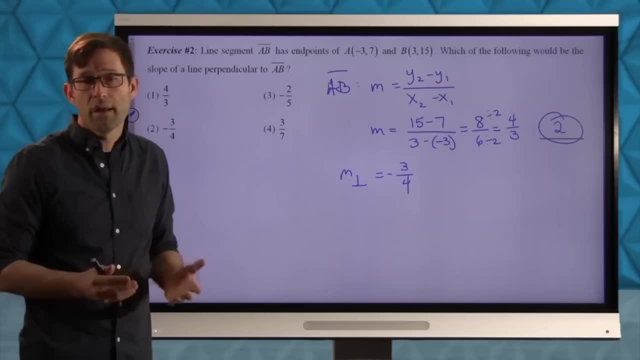 slope of a, b And piece number 2, what is the relationship of that slope, 4 thirds, with the slope of the line segment perpendicular to it? Negative reciprocals, Not hard right, You just got to take those two pieces of. 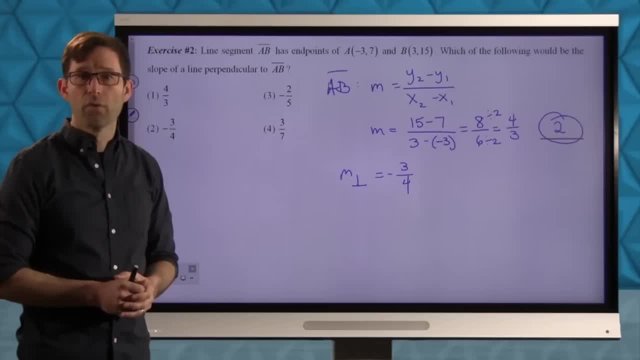 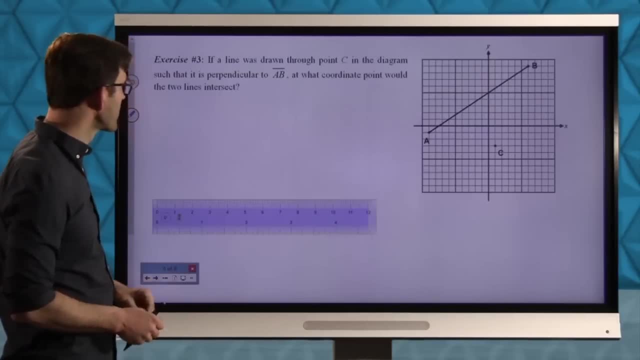 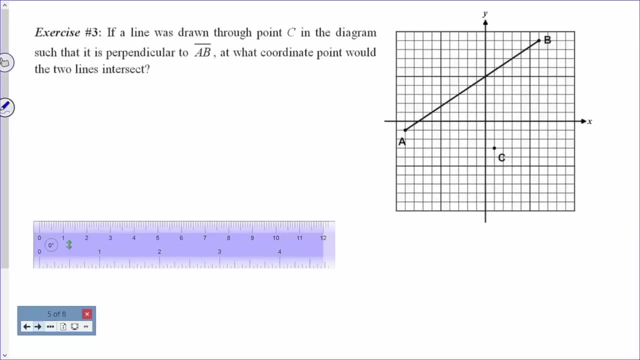 information together and work through the problem. Take a moment now, if you need to, to write down any part of this problem. All right, let's move on. Okay, slightly more challenging, but we've got a graph. Let's take a look. Exercise number: 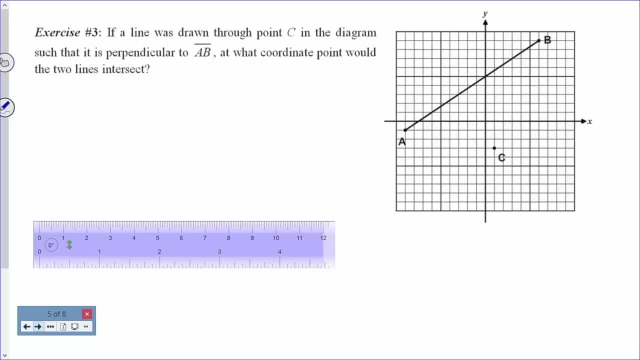 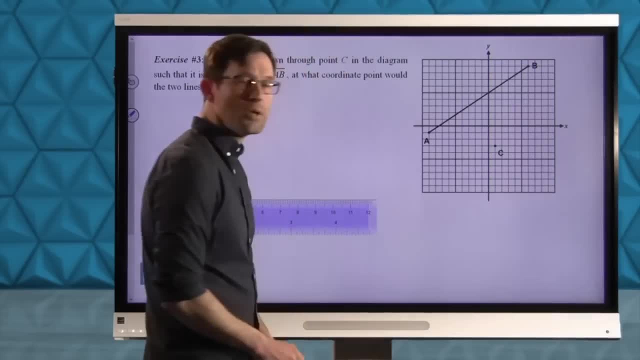 3. If a line was drawn through point C in the diagram such that it is perpendicular to a- b, at what coordinate point would the two lines intersect? So we've got this nice line, segment a- b, and we've got point C. I'd like to draw a line that goes through 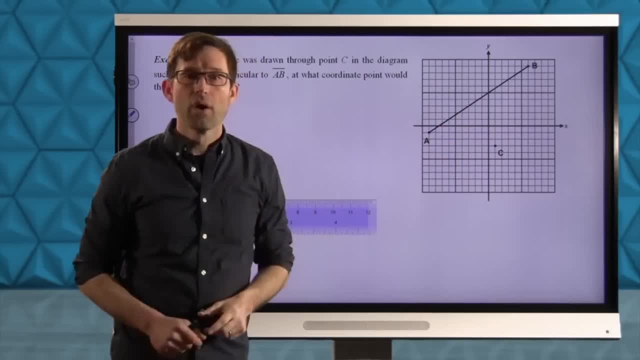 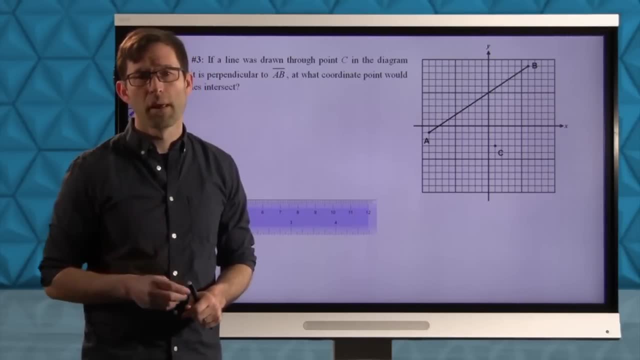 point C that is perpendicular to a, b, and I want to know the point where the two intersect. Okay, so again, this is challenging, but you have everything you need in order to be able to do this problem, and in those situations, I'd like 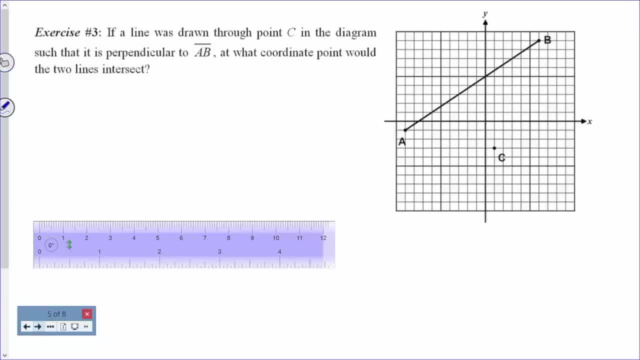 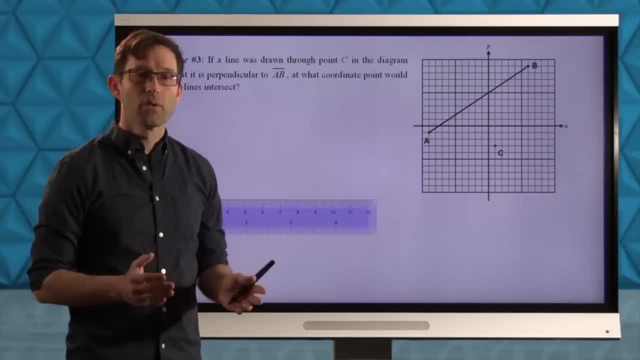 to take a moment and let you work on it. So go ahead and do so. All right, let's go through it. Well, what I'd like to do is I'd like to plot that line. I'd like to actually plot the line that goes through C. that's perpendicular. 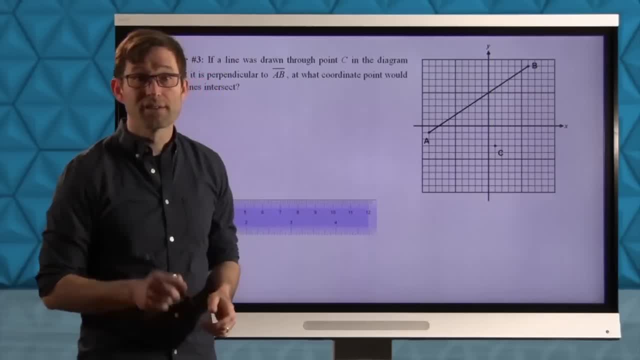 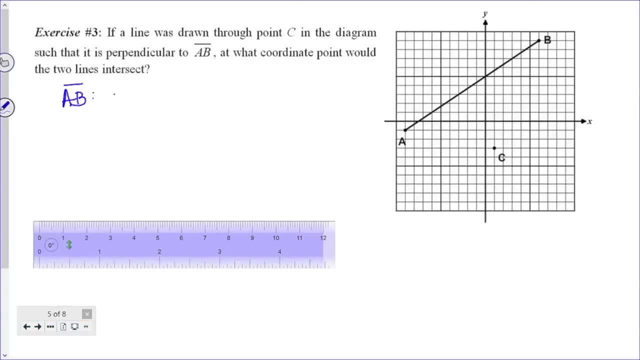 to a- b, but in that case I'd like to know what the slope of a- b is again, Just like the last problem. So let's do that Now. in this case, you could find the slope of a- b graphically, or you could find it algebraically, It's up to you, Since I've got the graph. 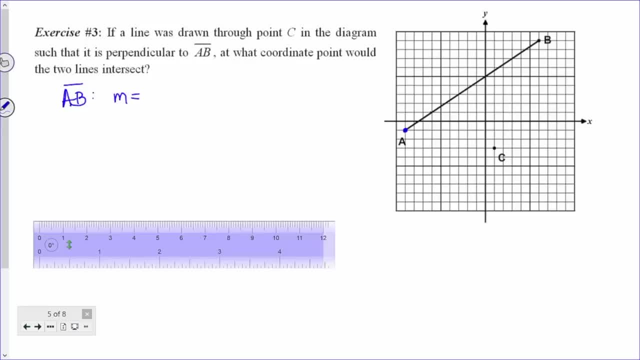 just sitting here, I think I'm going to do it graphically. So there's a nice point, a good point, a good point. I get the slope okay, So I can draw it graphically. Now let's good point, good point, etc. And it looks like the slope of AB is going to be a rise. 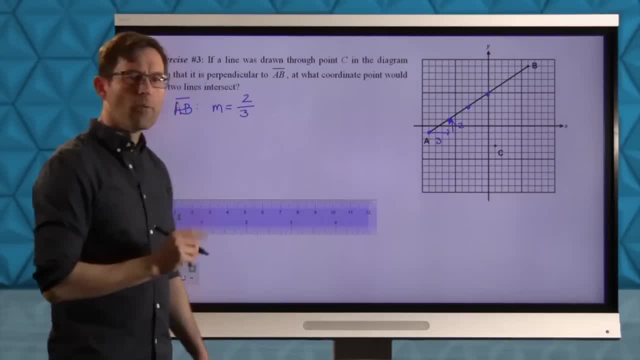 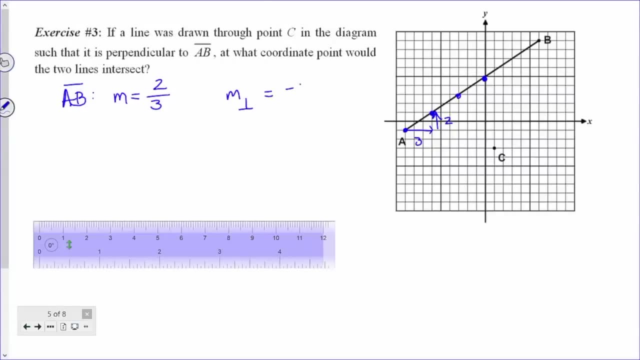 of 2 divided by a run of 3.. Now, what this tells me, though, is that the line that goes through point C will have to have a slope of negative 3 halves, meaning that it will have to fall. I'm still going to call it a rise by negative 3 and a run of 2.. So let's 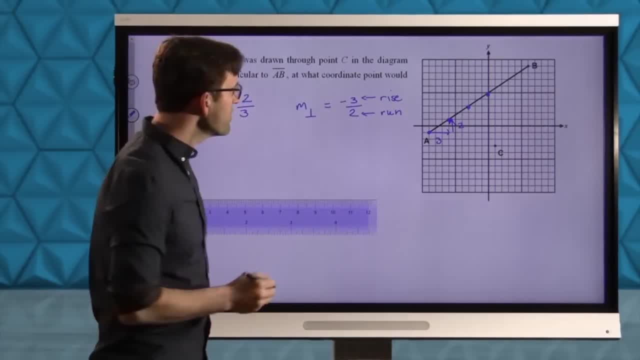 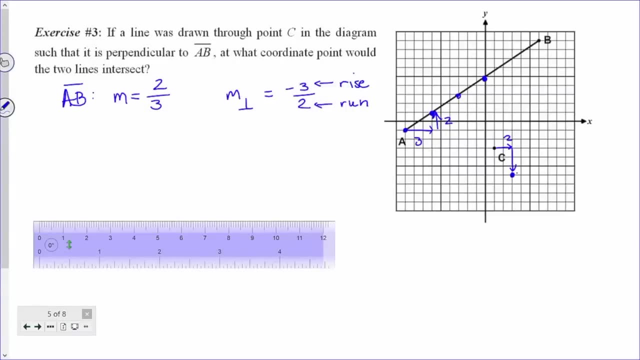 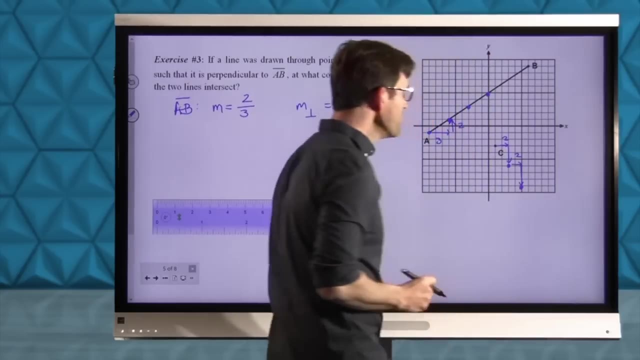 point. let's plot some points, okay. Specifically, let's go over to point C and let's go over 2 and down 3.. And over 2 and down 3.. Now, in a certain sense, this is a little bit unfortunate. 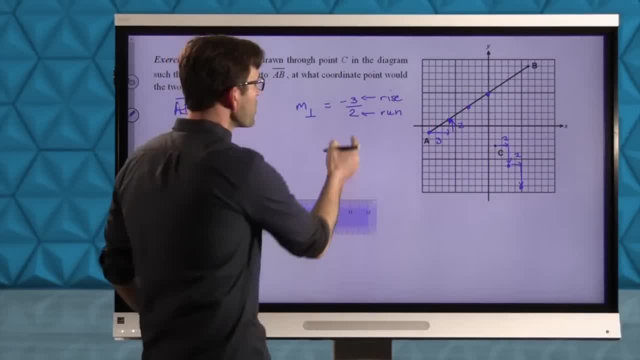 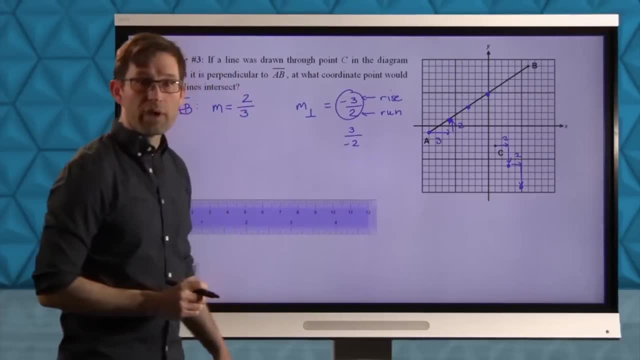 because it's going to be a run of 2 halves. But it's going to be a run of 2 halves, So we're going to be going in the opposite direction that we want to. But of course, we can interpret negative 3 halves as being negative 3 divided by 2, but we could also interpret it as 3. 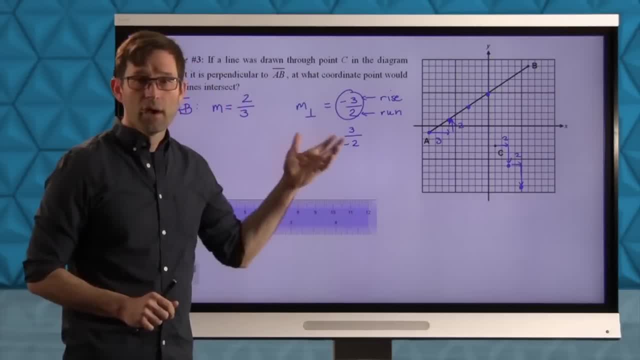 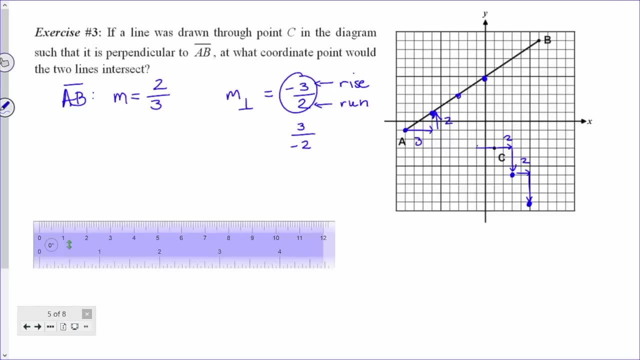 divided by negative. 2. Remember, a positive divided by a negative, a negative divided by a positive are both negative. In that case, what I'm going to do is I'm going to go to the left, 2 and up. 3. And I know you've done this before, when you've plotted lines And 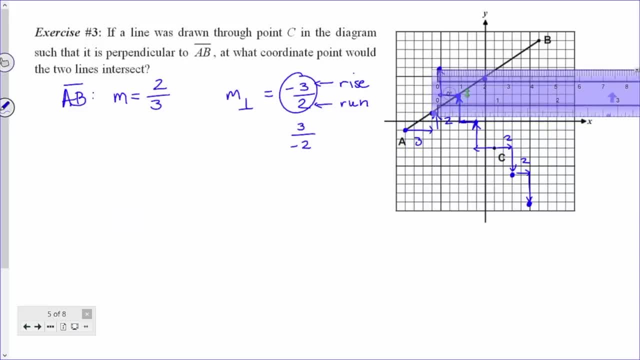 now what I can actually do is I can go ahead and plot the line. I think I'm going to do that. You can probably already see where the intersection is occurring. but let's get the line itself. There it is. And it's kind of nice too, because if you plot the line in it, 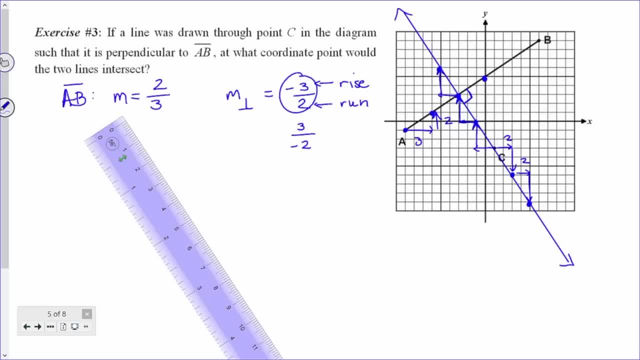 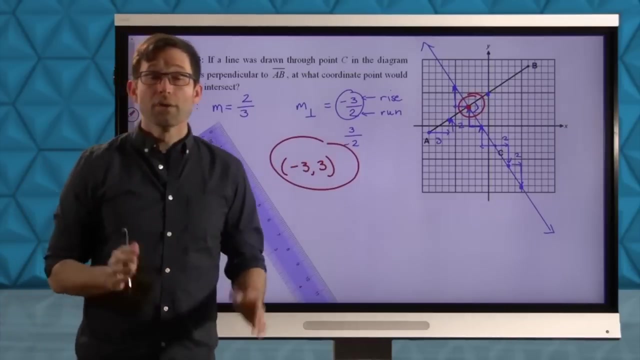 to me it's fairly obvious now that perpendicularity And of course the intersection point, And that is right here. So what are those coordinates? Looks like negative 3, 3.. Just making sure You bet Negative 3, 3.. That point right there, All right, So again it kind of ties everything. 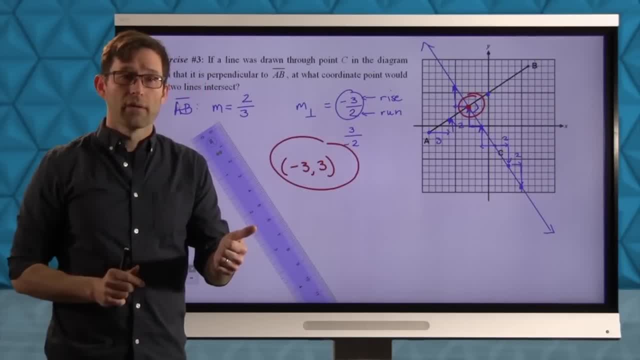 together, right? How do we find the slope of a line graphically? What is then the relationship between two lines that are perpendicular? Or what's the relationship between their slopes? Right, And then, of course, what's an intersection, The intersection point. None of this did we have to do algebraically, We didn't have. 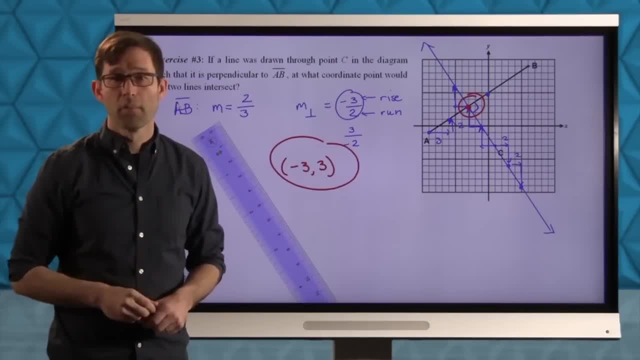 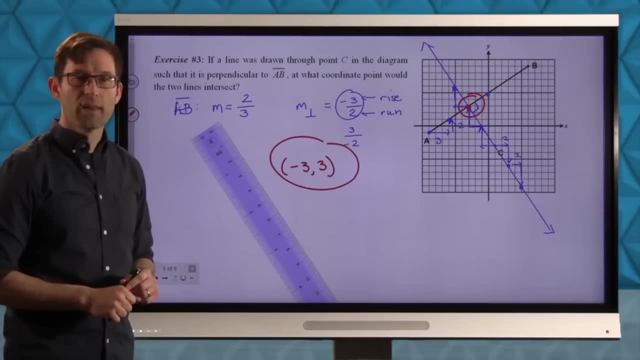 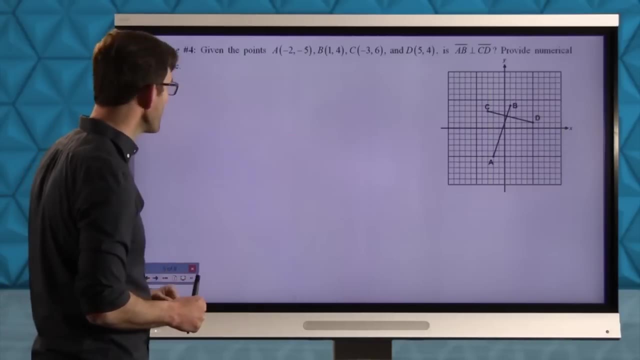 to set up any equation or anything like that. We just had to be able to plot that perpendicular line. All right, Let me step back for a second. Take a few moments with this, if you need to, And then we'll move on to the next problem. All right, Let's do it. Okay, Now we're getting. 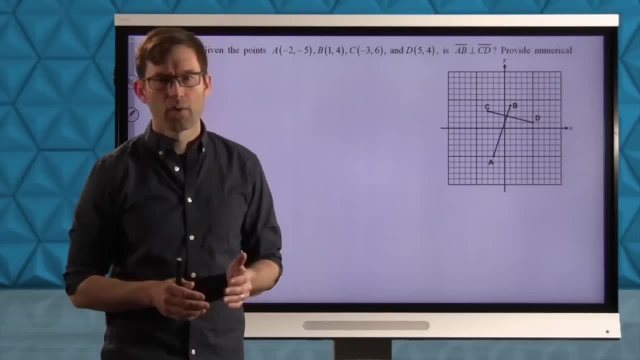 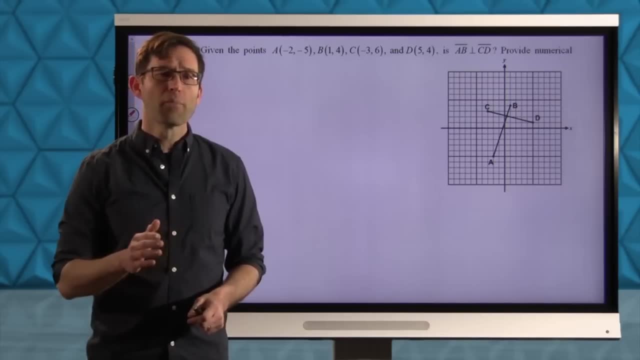 into the realm of what's called coordinate geometry proof. Okay, We looked at this a little bit with our parallelism. We're going to see it a lot more in the coming units because we want to be able to prove things not just using sort of like the Euclidean proof, you know, with side angle, side angle. 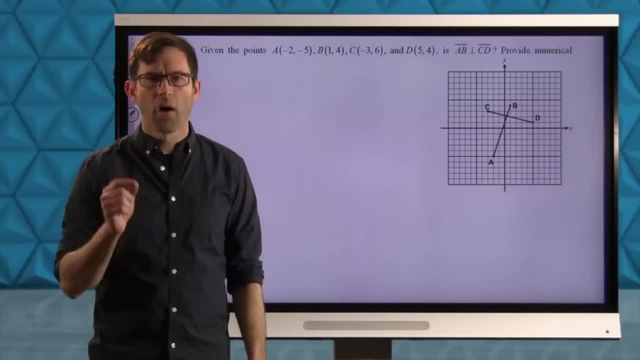 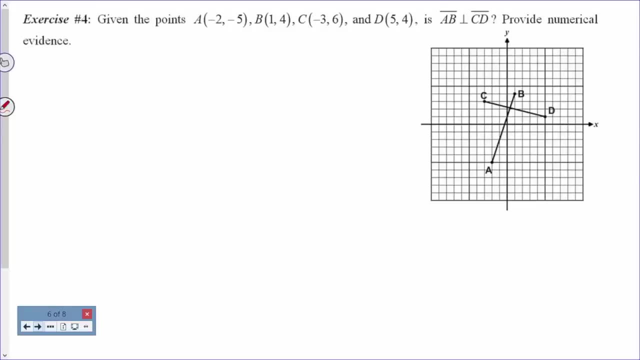 side angle, all that stuff. But we also want to be able to prove things with hard, solid numbers, And that's where coordinate geometry comes in. So let's take a look at exercise number four. Given the points A, B, C and D, I'll let you kind of read off their coordinates. 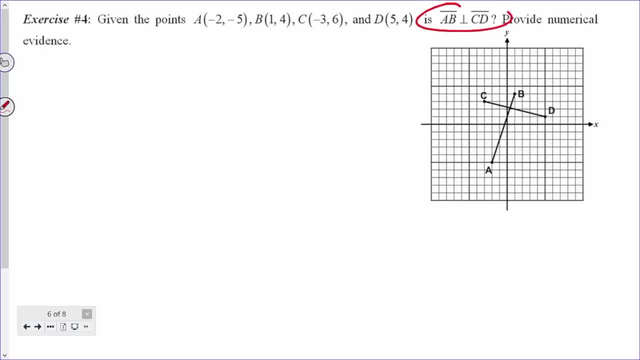 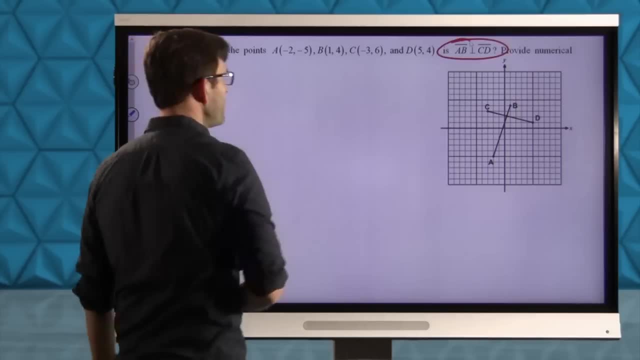 for yourself. Is A B perpendicular to C D? I'm going to give you a little bit of a hint. I'm going to give you a little bit of a hint. Is A B perpendicular to C D? Provide numerical evidence, All right. Well, when we look at, 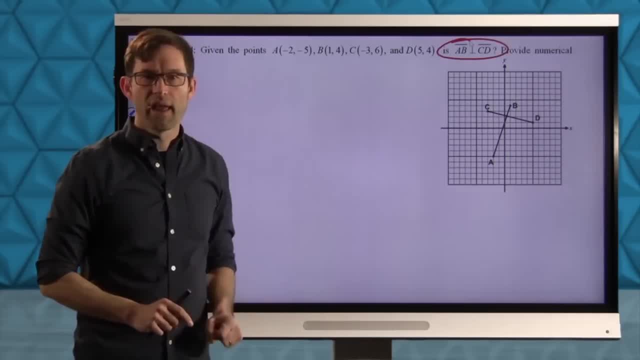 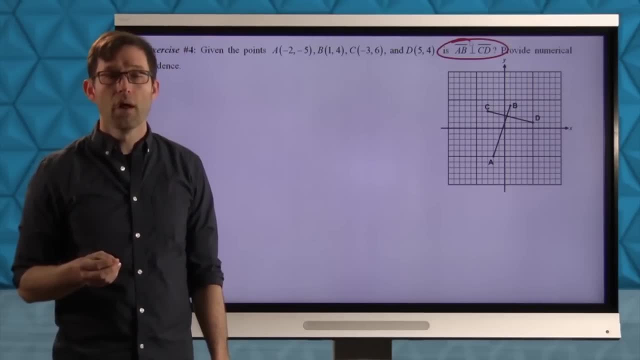 the picture it certainly looks like it's possible that A- B is perpendicular to C- D, But the ultimate test is not whether it looks like the two segments are perpendicular, but whether or not their slopes are negative reciprocals. So what I'd like you to do is 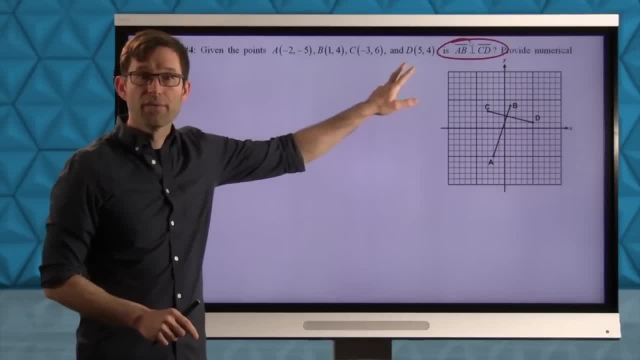 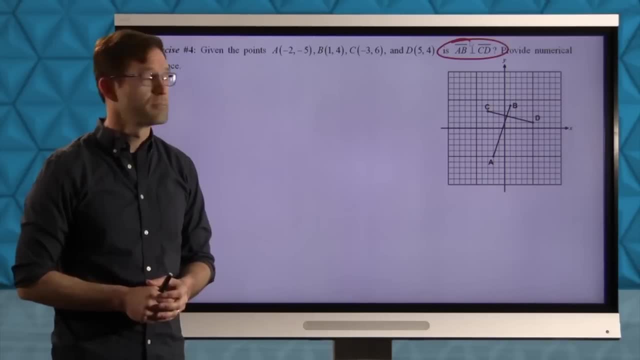 take a few minutes to calculate the slope of A, B and to calculate the slope of C, D. make the comparison and then we'll see what happens. Okay, So let's take a few minutes And then make the call. Are they perpendicular? Take a little bit of time. 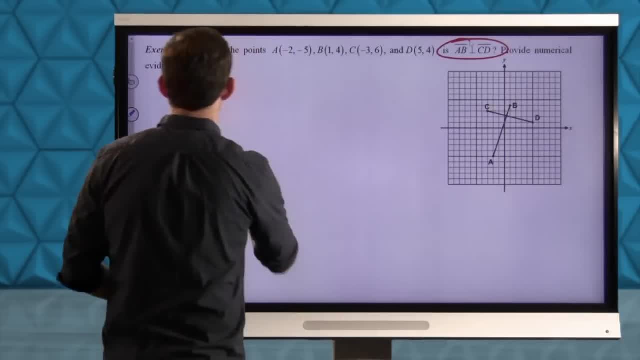 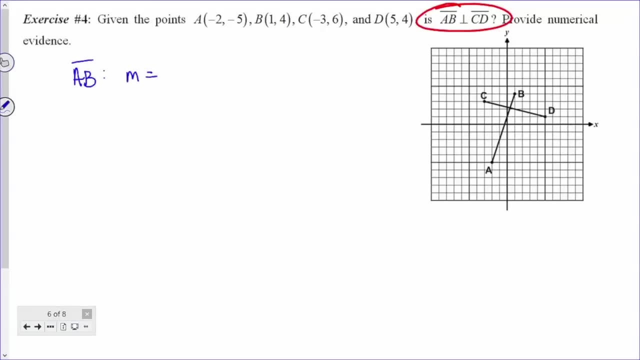 Okay, Let's go through it. I'm going to go just straight up with the slope formula. Now you do have the graph sitting there. You could possibly do it graphically, But let's do A, B right For its slope. we'll do four minus negative, five all divided by one minus negative. 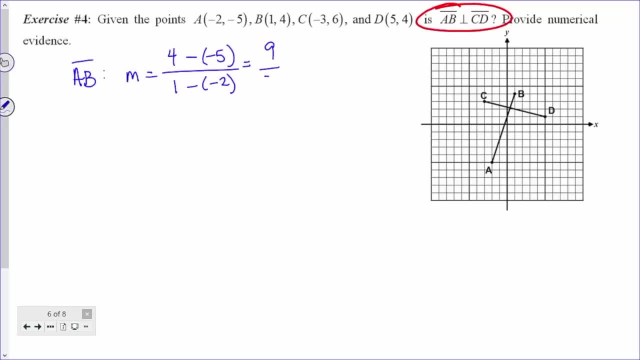 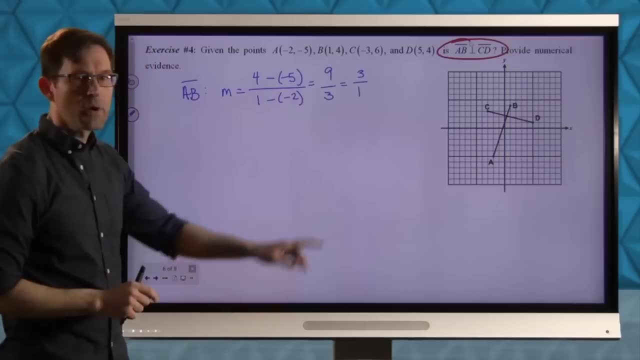 two. Okay, and in the numerator that leaves me with nine, and in the denominator it leaves me with three, And I could reduce that to three, or I can reduce it to three over one. I think I'm going to reduce it to three over one because I'm looking for that negative. 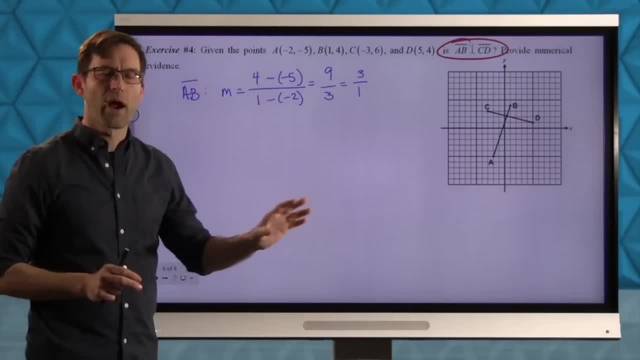 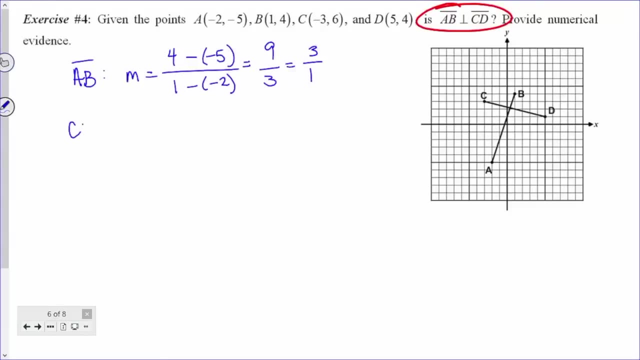 reciprocal business. So having the slope written as a fraction as opposed to a whole number is helpful, at least in this context. Let's now go through C D. All right, For C D, my slope is going to be four minus negative five. I'm going to take a few minutes and 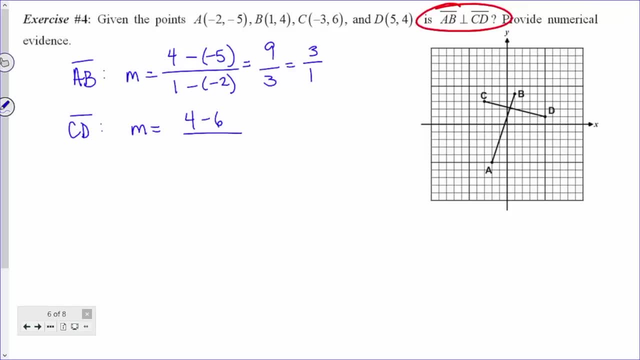 see what happens. Okay, So for C D, my slope is going to be five minus negative, three, 4 minus 6, all divided by 5 minus negative 3.. Watch those double negatives: 4 minus 6 is negative, 2.. 5 minus negative, 3 is positive, 8.. 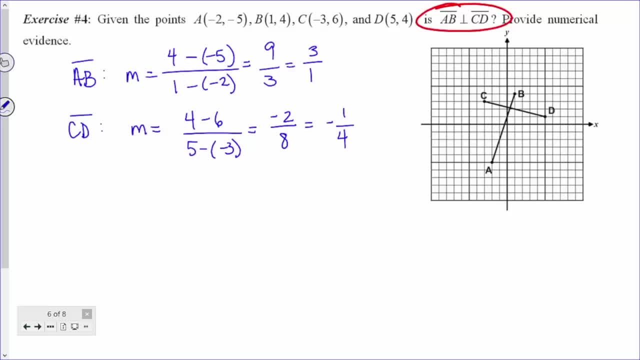 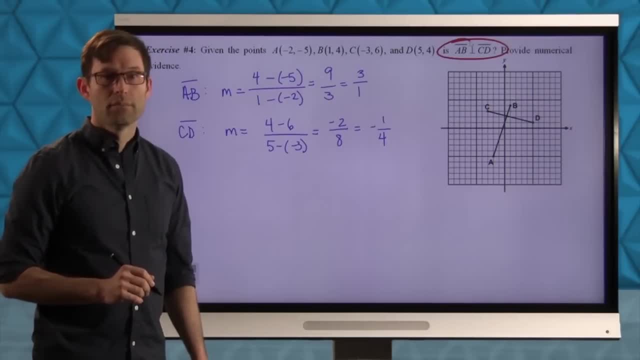 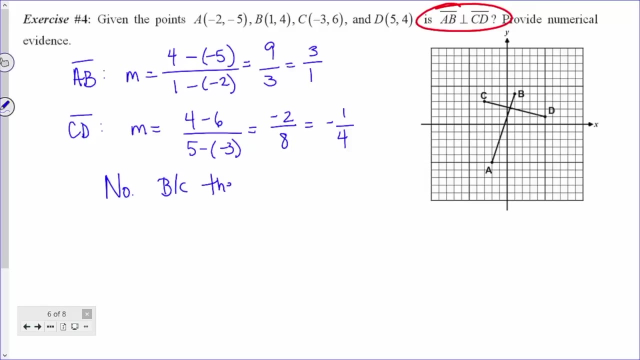 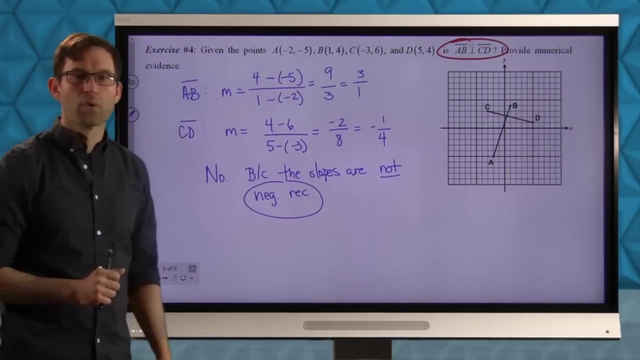 Again, it pays to reduce and we get negative 1. fourth, So are they perpendicular to each other? And the answer is no. No Why? Because the slopes are not negative reciprocals. By the way, this is a very, very common way to sort of abbreviate that phrase. 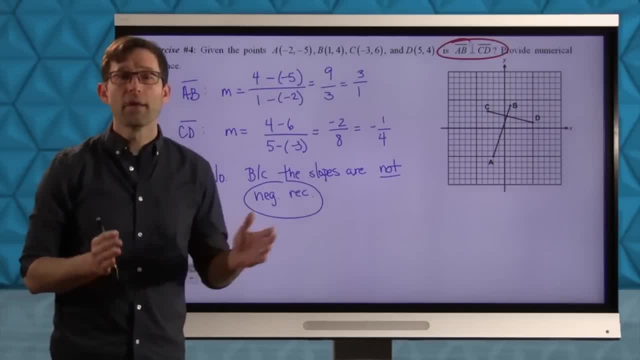 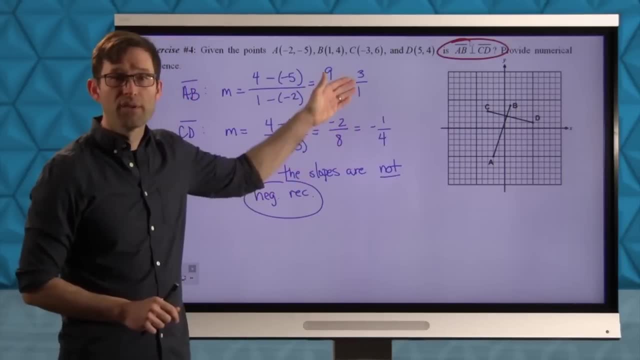 negative reciprocals. You could certainly do it Again if your teacher would like you to use that idea of the product being equal to negative 1, you could do that. For instance, if I actually did the product of these two slopes, it would be. 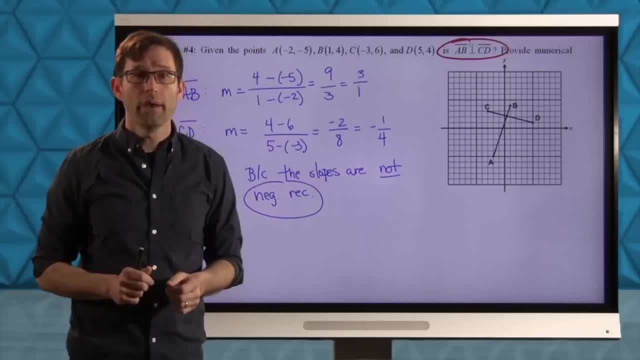 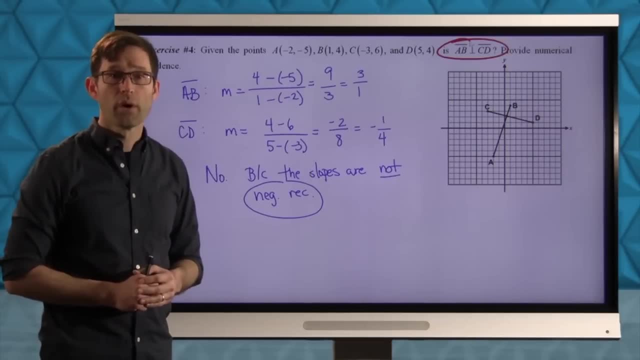 negative 3 fourths, Which obviously is not equal to negative 1.. But I'm going to pretty much primarily stick with the idea of being able to recognize whether two numbers are negative reciprocals of one another. and they're not. By the way, they're pretty close. Just for the record, they're pretty close. 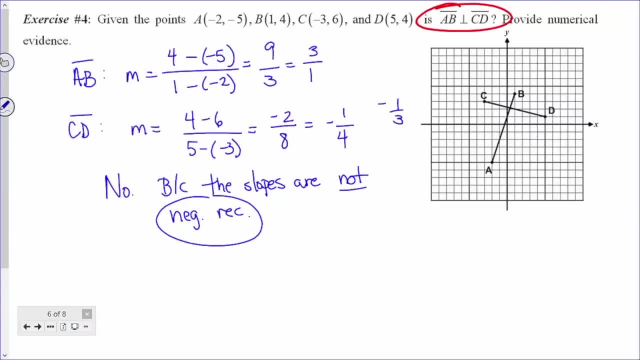 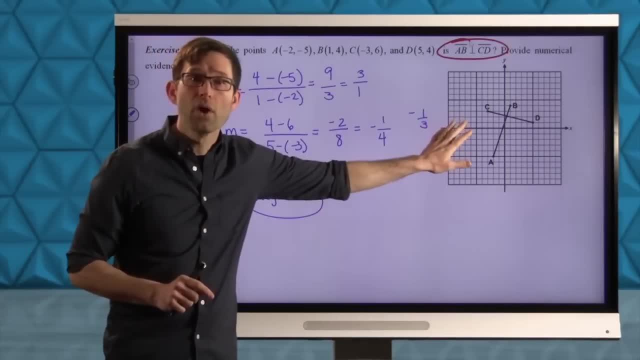 Had this thing turned out to be negative 1 third, which is obviously a fraction very close to negative 1 fourth, then they would have been perpendicular, And that's why they look very close to it up here. They look close to it because their slopes are close to being. 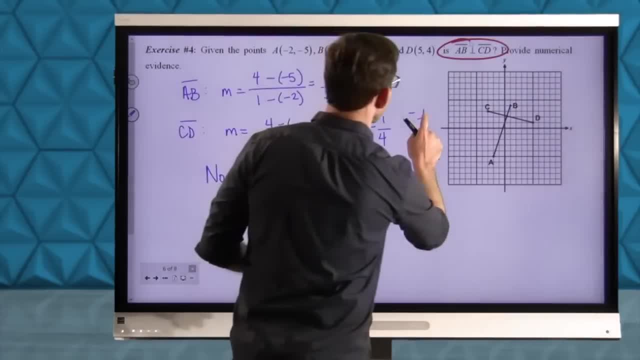 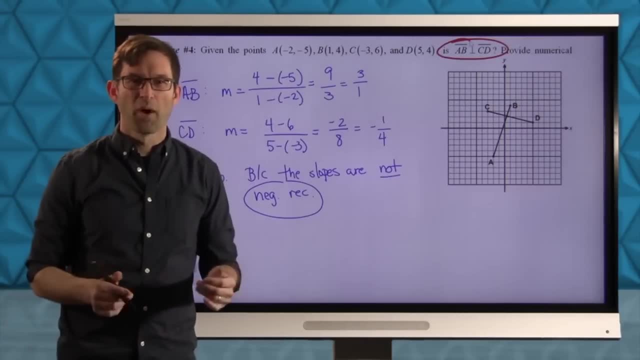 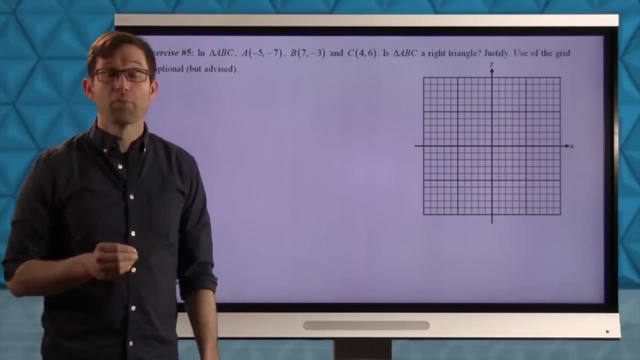 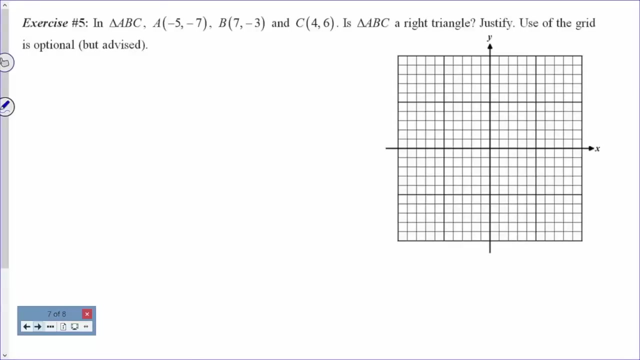 negative reciprocals. They just aren't quite Whoops, So let's get rid of that. All right, Let's do one more problem. The last piece is to determine whether or not a particular triangle is a right triangle Right. So in exercise number 5, it says: in triangle ABC A is negative 5, negative 7,. 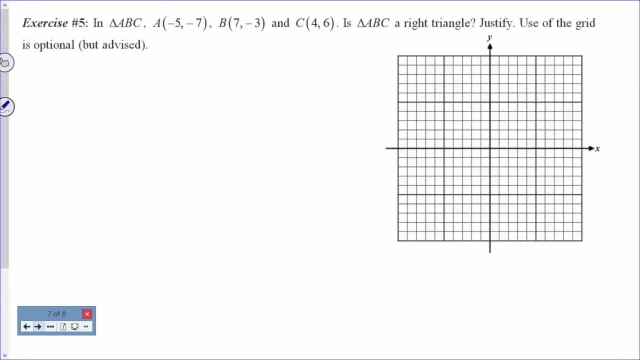 B is 7, negative 3,. C is 4, comma 6.. Is ABC a right triangle? Justify? Use of the grid is optional but advised. OK, You'll see that terminology on a lot of standardized exams where they give you. 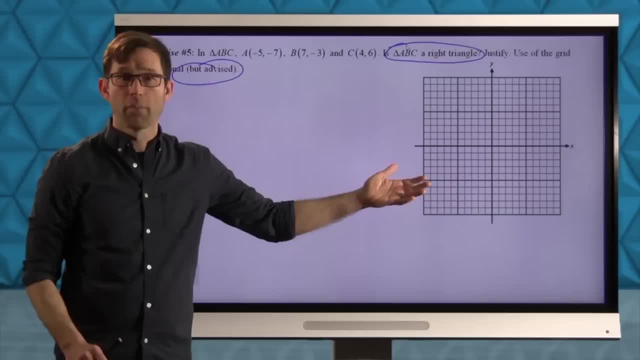 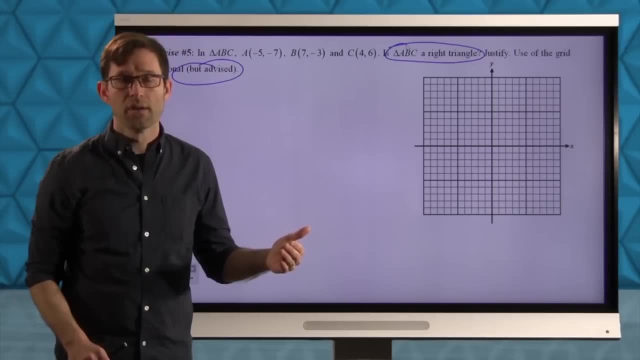 a piece of graph paper within a problem and they say: well, you can use the graph paper if you want, but you don't have to. It's almost always the case that if they've given you graph paper, then it's a good idea to use it, but it's not all absolutely necessary. 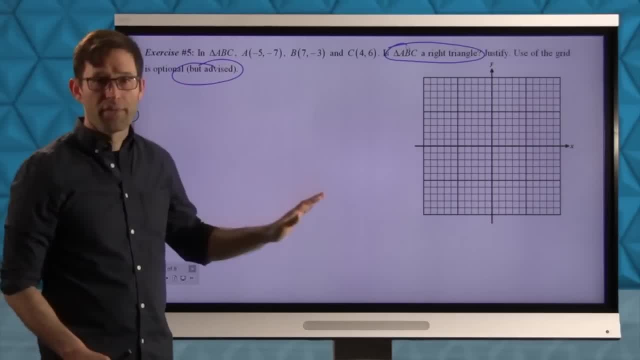 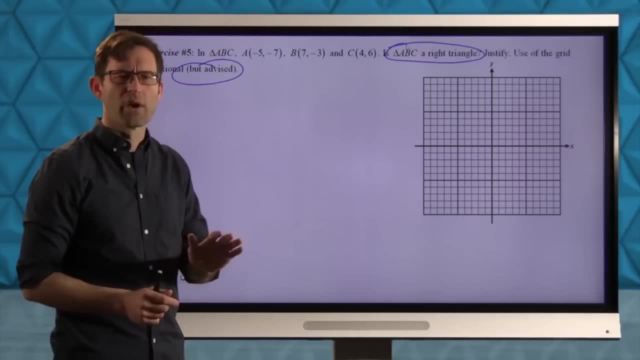 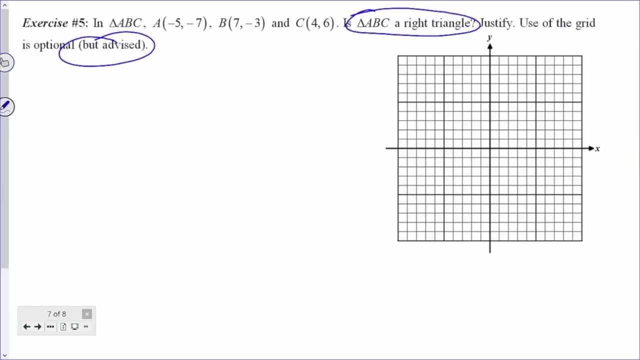 OK, Now I assume you can plot these things. OK, But pause the video now. Take a couple of minutes and plot that right triangle. Oh, I'm sorry, Plot that triangle. We're trying to determine if it's a right triangle. 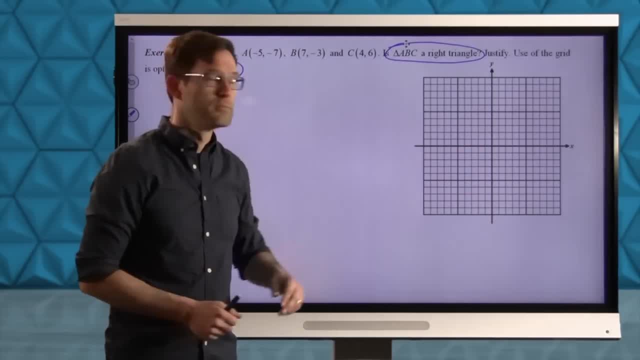 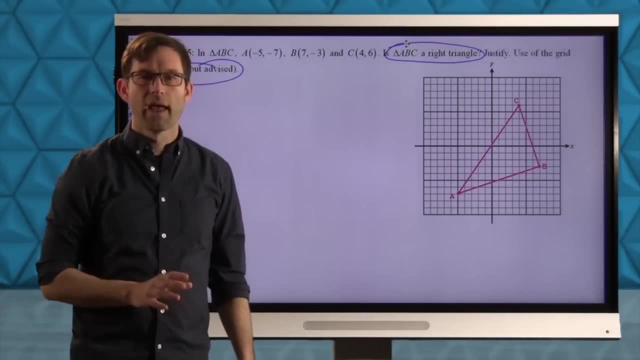 You haven't plotted, Because I'm just going to make it magically appear. Well, I was going to make it magically appear There, it is All right. Anyway, there's my triangle, OK, And I'm trying to determine whether it's a right triangle. 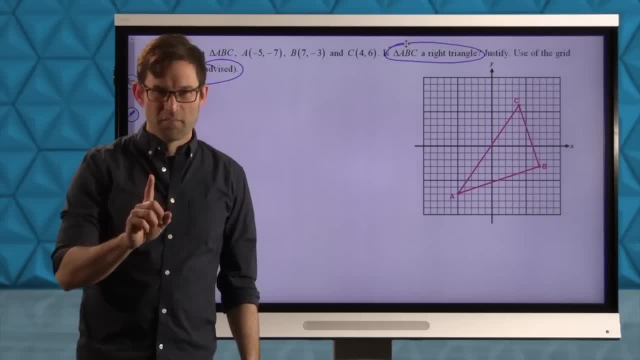 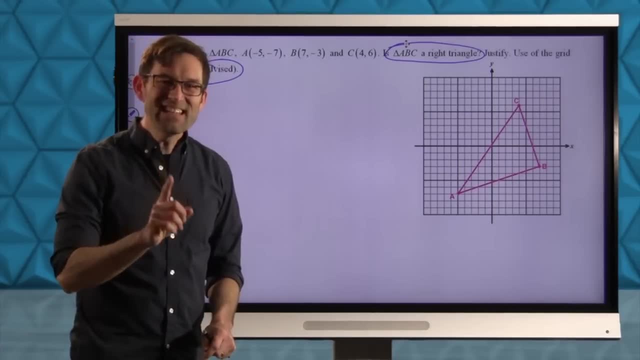 Now let's talk about why the use of the grid is optional, but advised. OK, This triangle certainly looks like it could be a right triangle, But if it is a right triangle, if it is a right triangle, the only way that's. 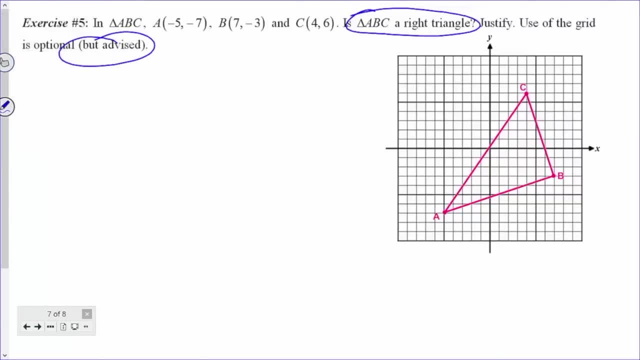 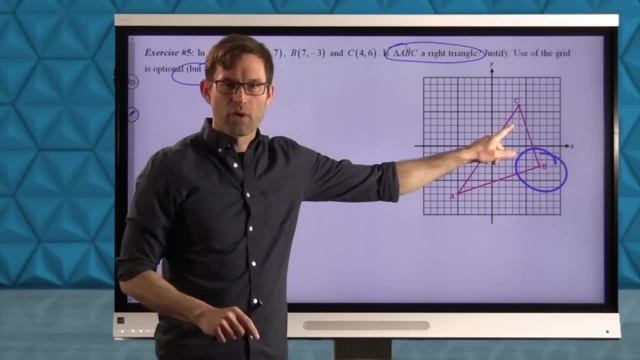 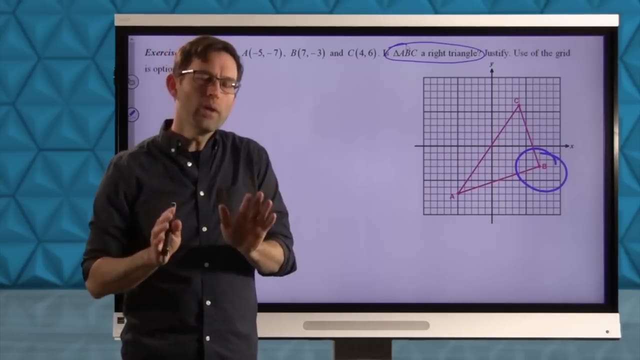 going to happen is if this angle is a right angle. There's no way that that's a right angle or that's a right angle. So if my plotting is correct, if I haven't made a mistake in my plotting, then really what I want to see is whether or not this line segment is a 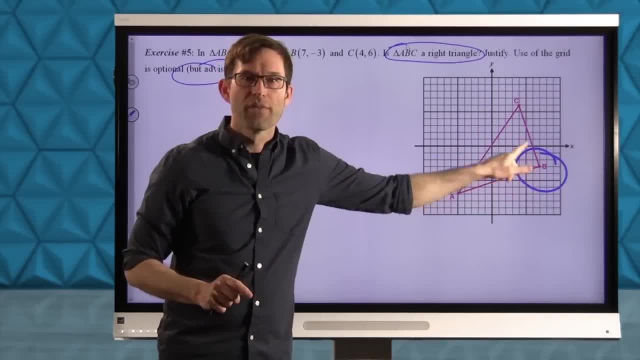 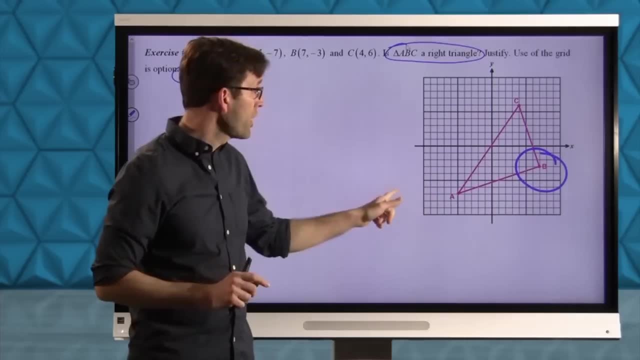 perpendicular to this line segment, which is AB, is perpendicular to this line segment, which is BC. OK, That's what I'm trying to do, So I can lessen my work. Could I also calculate the slope of line segment AC? Sure, I could. 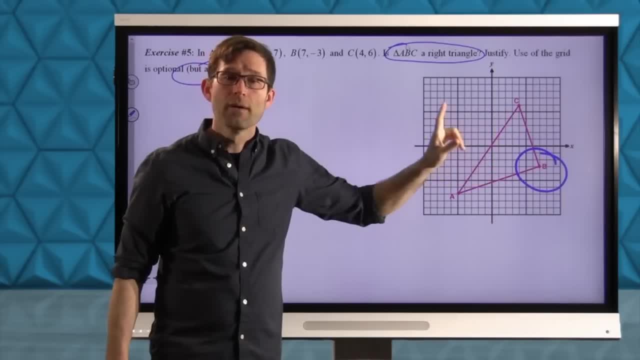 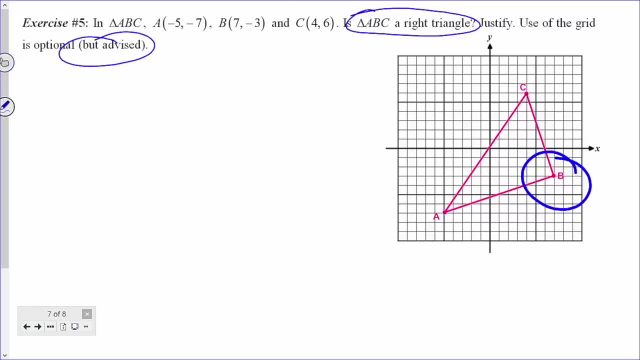 And in some situations we're going to want all three slopes, But here let's just do the slope, Let's just do the slope of AB, And let's just do the slope of AB And let's just do the slope of AB. 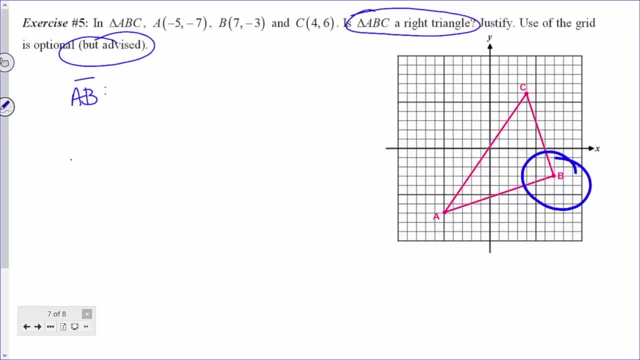 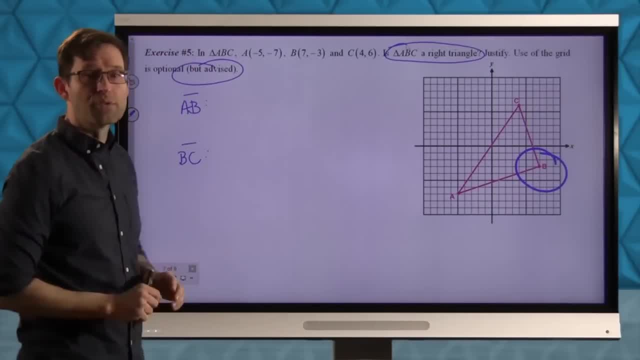 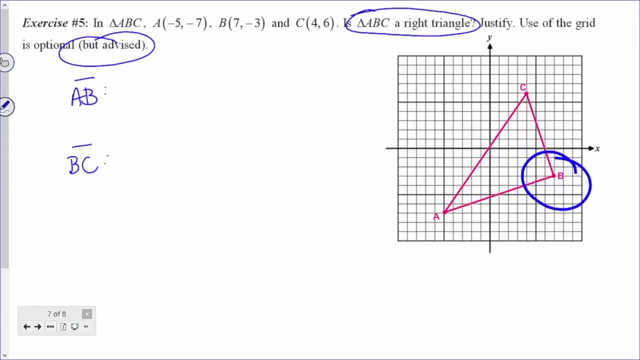 Why don't you take a few minutes, calculate those two slopes, then make your decision about whether or not this is a right triangle? OK, Let's go through it. Here we go. AB: Negative 3 minus negative 7, all divided by 7 minus negative 5.. 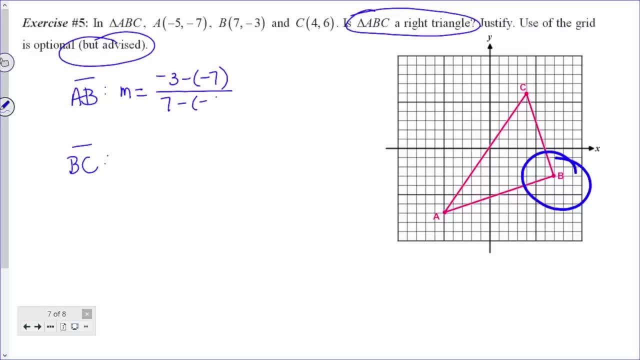 All right. So let's just do the slope of BC. OK, Let's just do the slope of BC And let's see. So here is negative 3 minus negative 5. Negative 3 minus negative 7.. Watch out, that could be a tricky one. 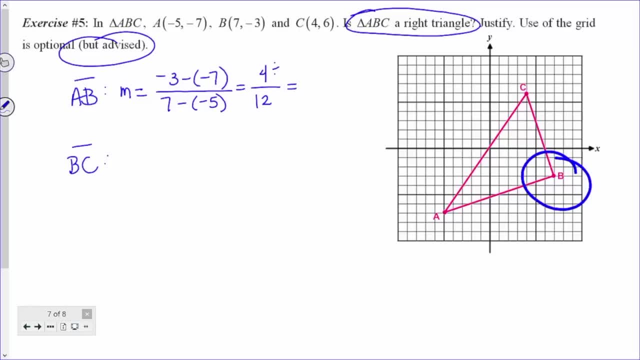 It's positive 4.. 7 minus negative 5. That one's easy. Positive 12.. Again, I'm going to reduce by dividing both numerator and denominator by 4. And I'm going to find that slope of AB is 1. third, 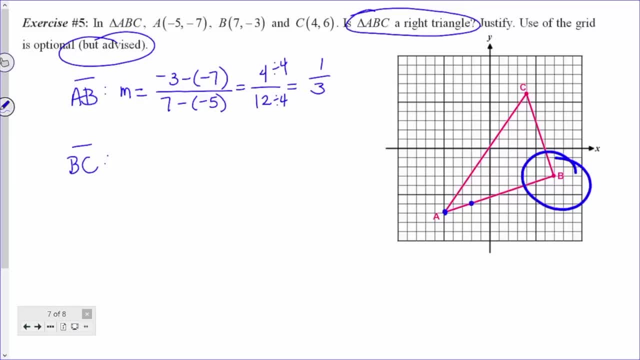 By the way, it also doesn't hurt to then graphically check that If I came over to line segment AB, I could easily then see: right, I rise 1 unit, So that slope of 1 third makes sense. Let's do BC Alright. in BC, the slope. 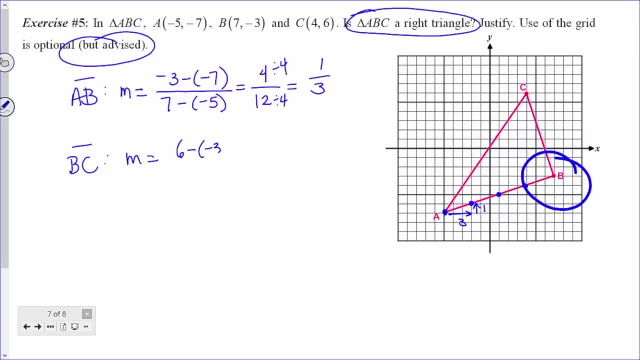 is going to be 6 minus negative 3, all divided by 4 minus 7.. Okay, 6 minus negative 3 is 9.. 4 minus 7 is negative 3. And if I divide both of those by 3, I get negative 3 over. 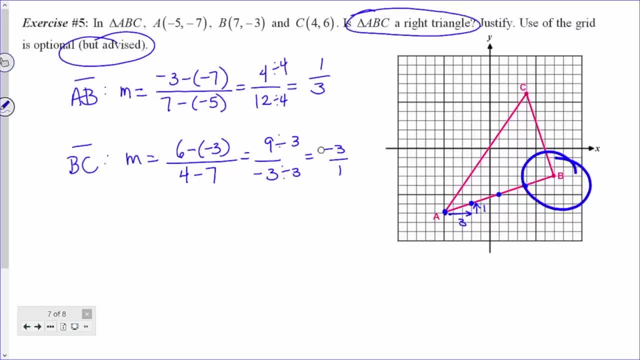 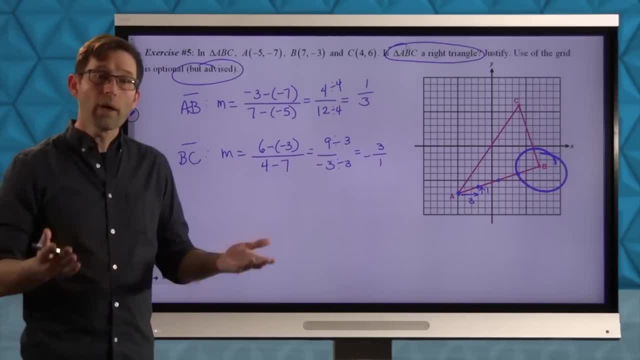 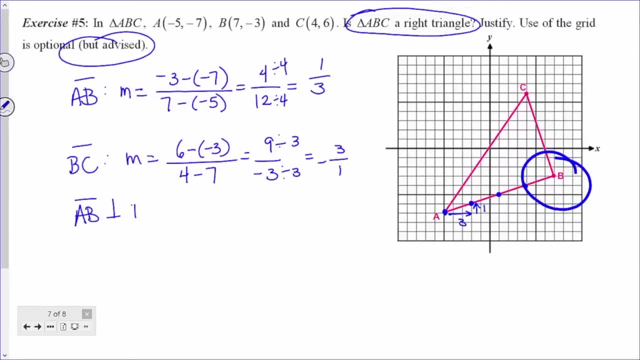 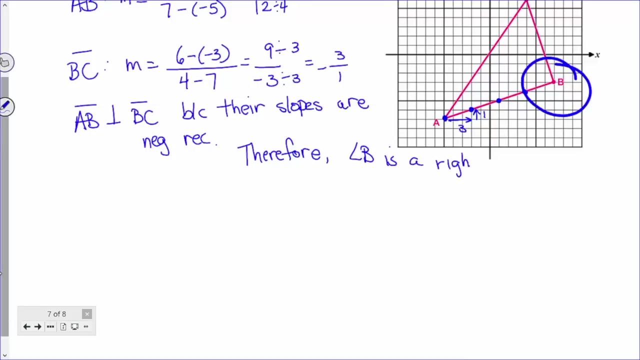 1. Or, better yet, how about I just get negative 3 over 1.. Okay, so what can I now say, right? Well, I can now say that AB is perpendicular to BC Because their slopes are negative reciprocals. Therefore, angle B is a right angle. 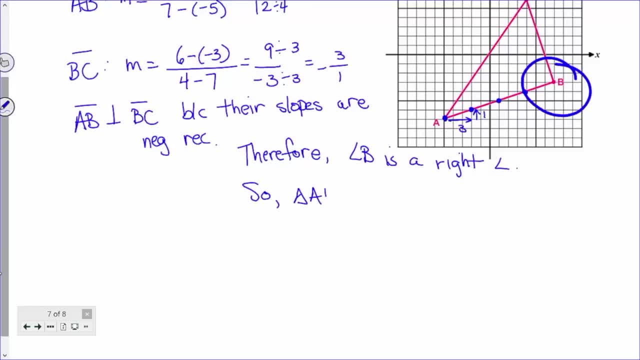 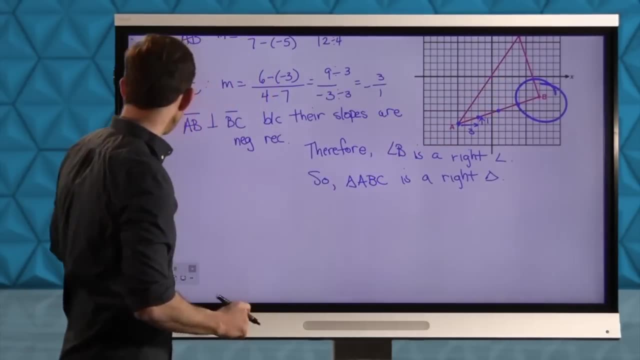 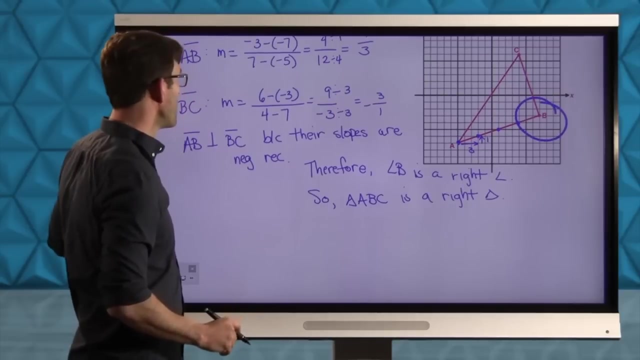 So triangle ABC is a right triangle. Look at the logic there, right, These two sides right are perpendicular. Let me bring this picture up a little bit. So side AB and BC are perpendicular and we know that just based on their slopes: Slope of positive, 1 third, a slope of negative. 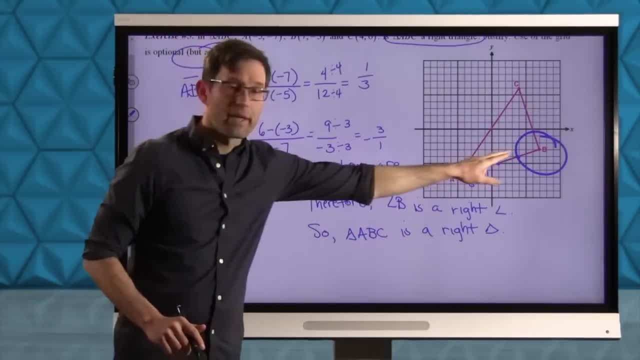 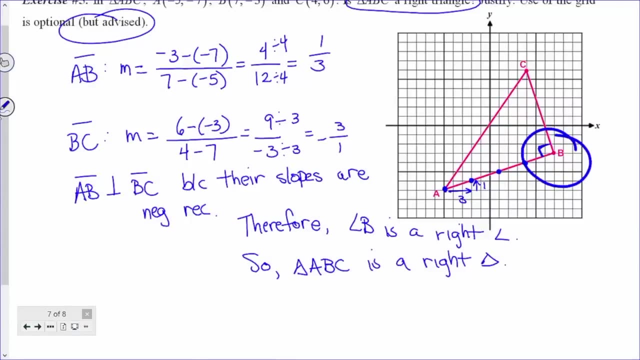 3. Okay, Because they're perpendicular, I can say that angle B is a right angle. Let me mark that just so that you kind of see it on there. That's now a right angle And because that's a right angle, triangle. 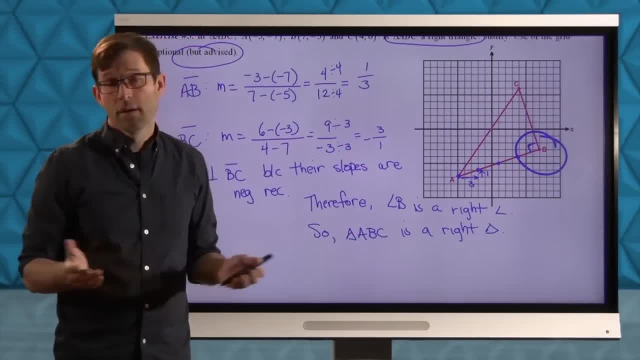 ABC is a right triangle, Alright, And that's a very, very simple coordinate geometry proof. Don't get me wrong: the last one we did was also a coordinate geometry proof, Alright, And they both involve the same thing, which is, were two line segments perpendicular to 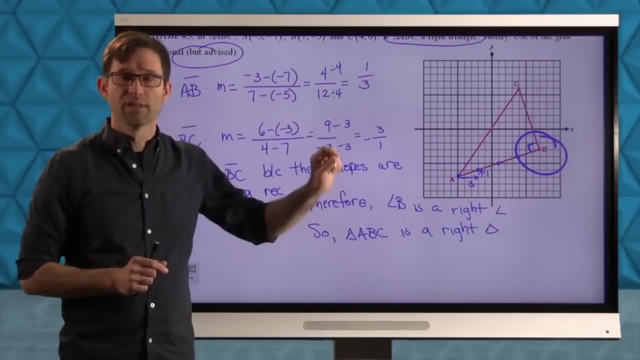 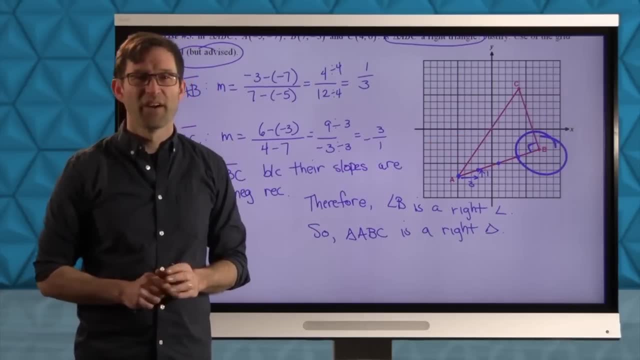 each other, But this one got to a bigger picture, which is: can we then, you know, say something about that perpendicularity in terms of the triangle that we have plotted here? Alright, Let's wrap this lesson up. So, in the first lesson of this unit, we saw that 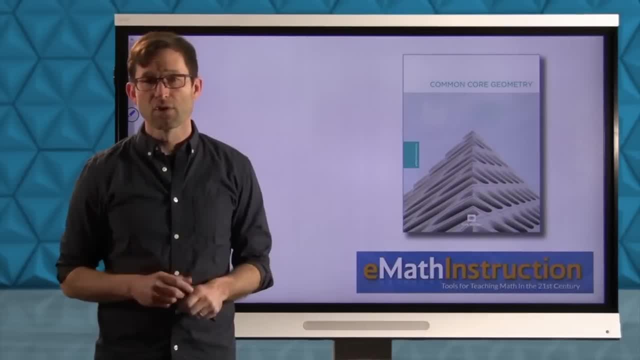 when two line segments have equal slopes, those line segments are parallel. Just as important as parallelism, though, is perpendicularity. when two lines or line segments form 90 degree angles, There the slope relationship is more challenging. The slopes are negative reciprocals. 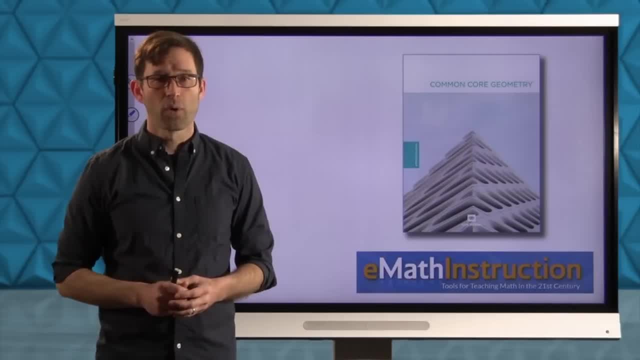 So if one of them is 4, fifths, the other one is negative, 5 fourths. If one of them is 7, the other one is negative, 1, seventh, Okay, But using that relationship you can solve a lot of problems that are very similar to the ones that we did with parallelism. Right. 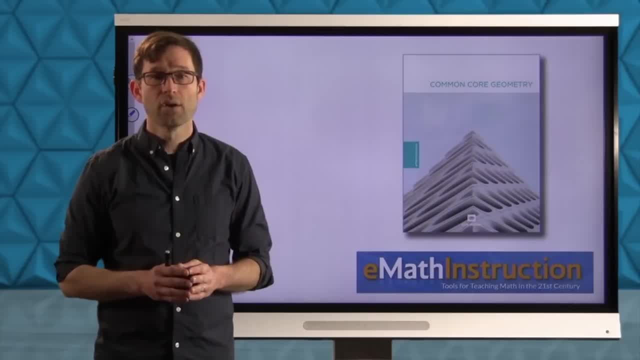 Whether that's, you know, sort of like finding out where two lines intersect or determining whether a triangle has a right angle in it. Okay, Again, we're going to need this a lot when we get into things like squares and rectangles, in which right angles serve a very, very critical role. 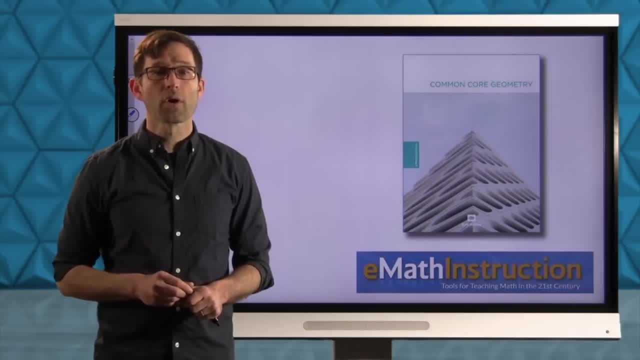 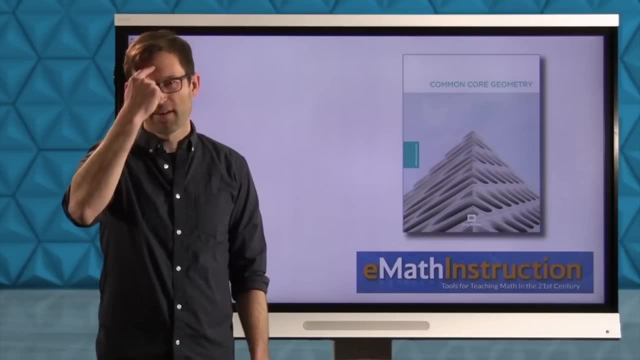 For now, though, I'd like to thank you for joining me for another Common Core Geometry lesson by E-Math Instruction. My name is Kirk Wyler, and until next time, keep thinking and keep solving problems.